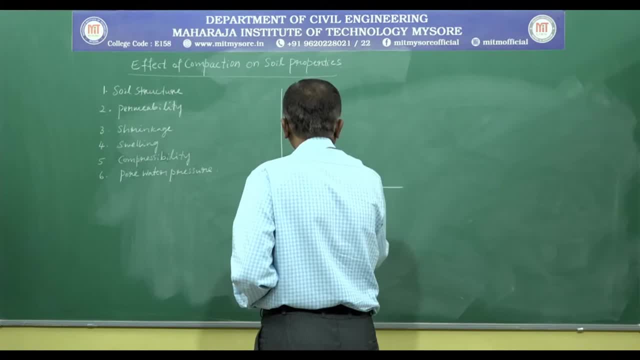 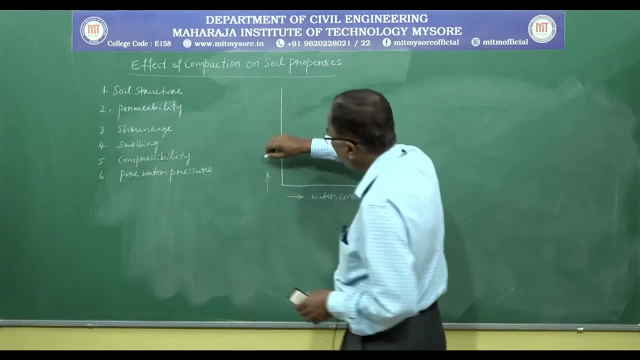 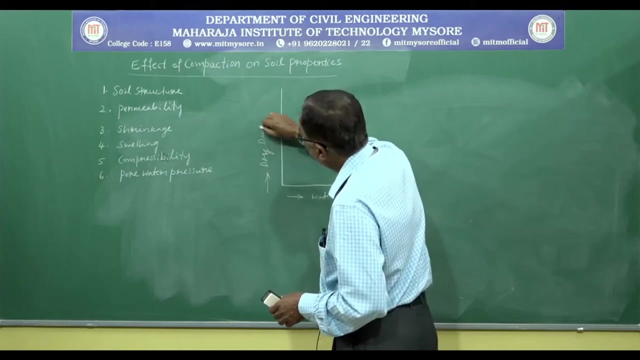 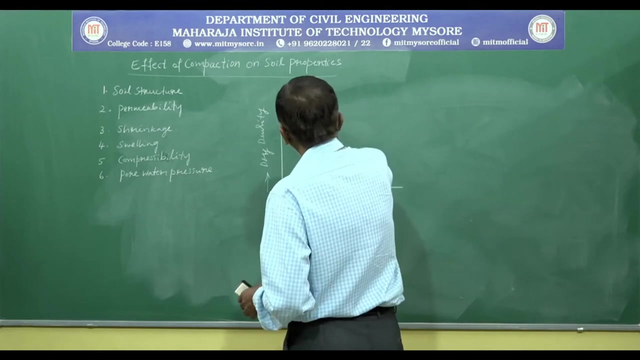 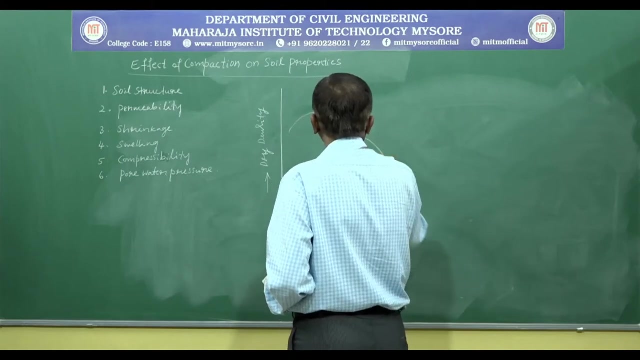 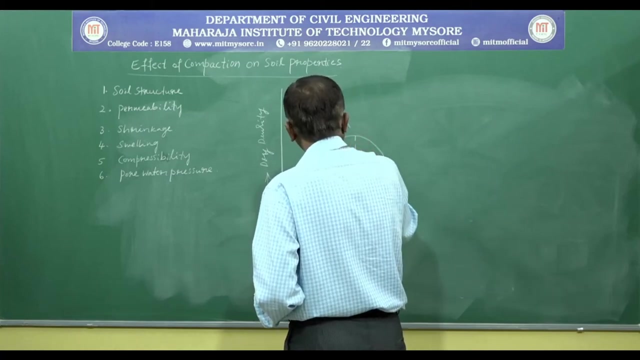 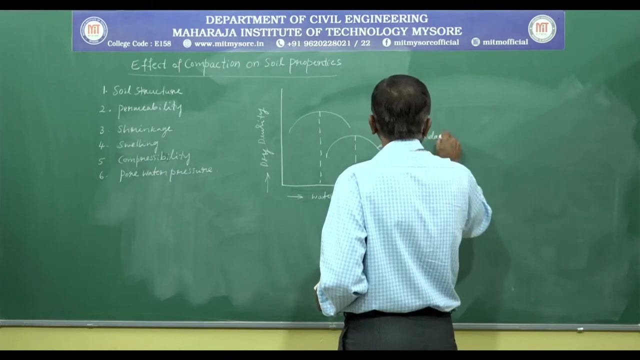 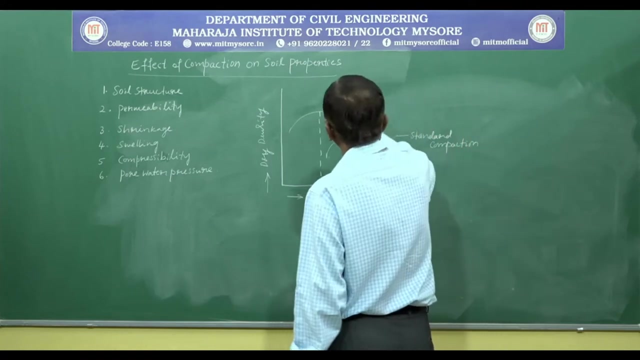 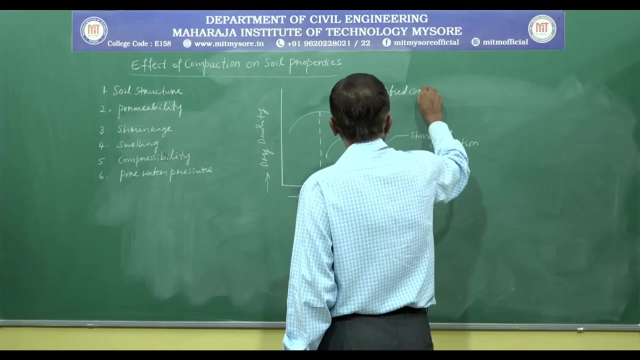 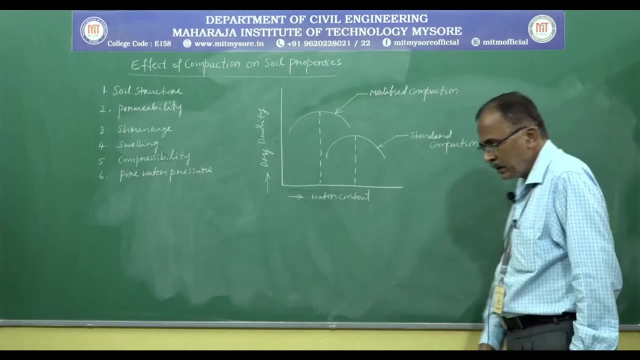 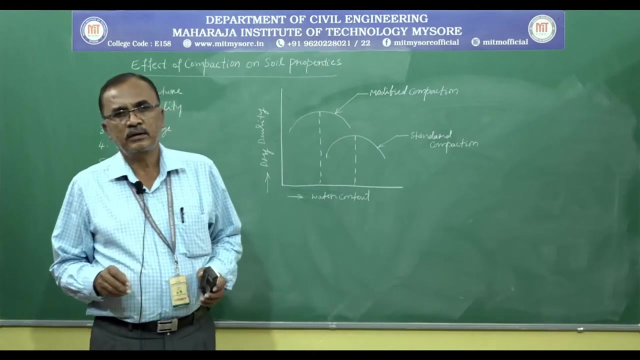 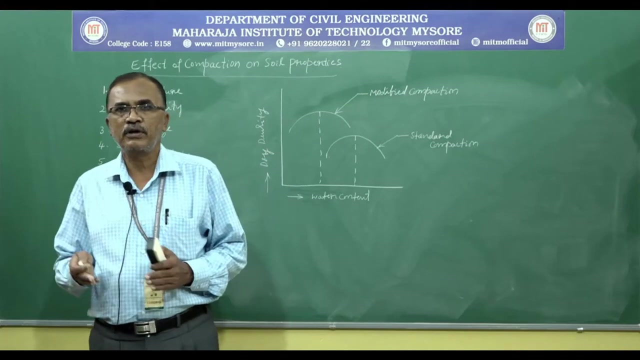 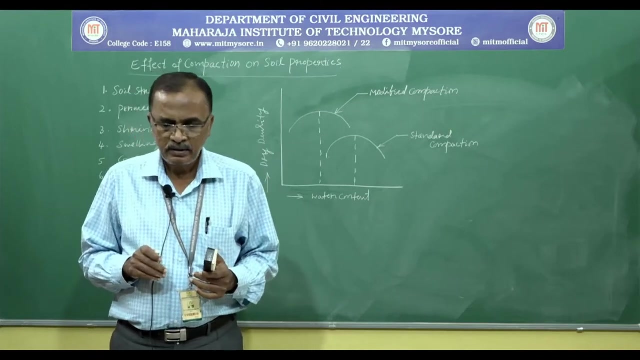 For that we have considered a standard compaction and modified compaction In soil structure. we discussed that in disturbed soil dispersed structures are predominant. That is in case of cohesive soil. In cohesion less soil particles are not in contact with each other. 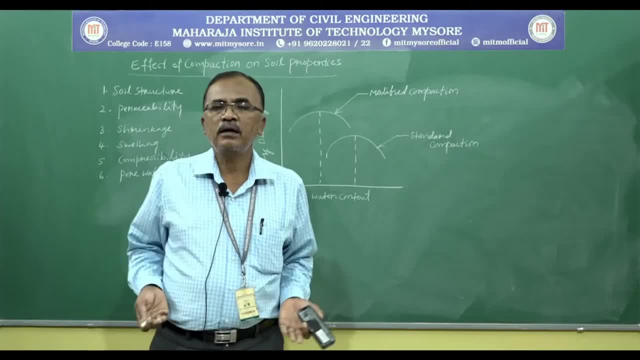 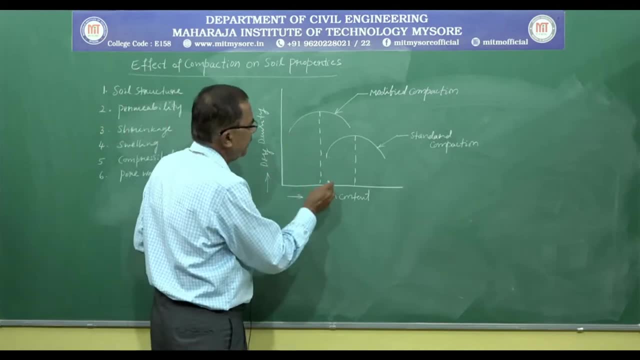 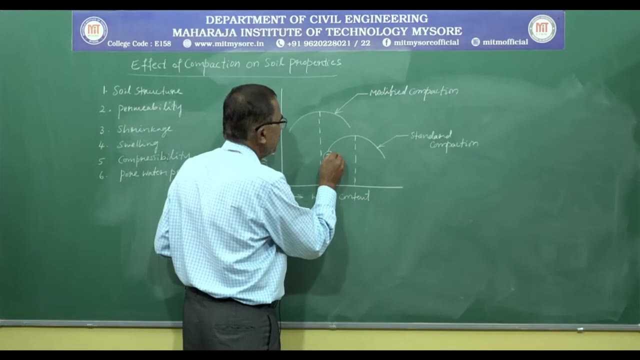 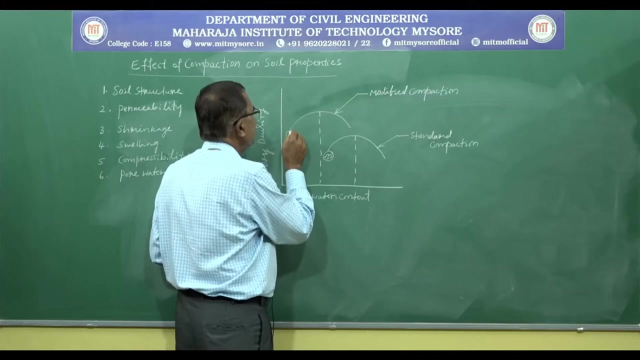 And sometimes they are in honeycombed structures. Say, for example, that you can understand like this: To begin with, the orientation of particles will be like this: almost the parallel orientation, face to face or edge to edge orientation. we can see like this: Ok, 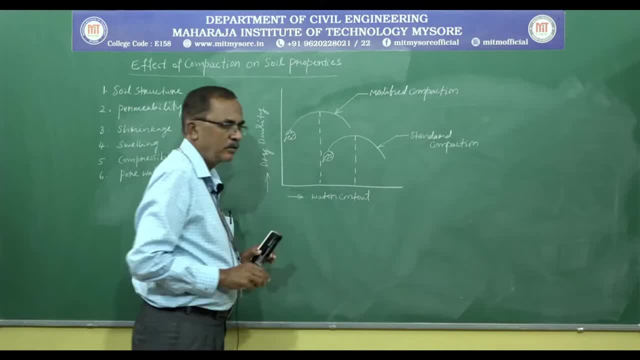 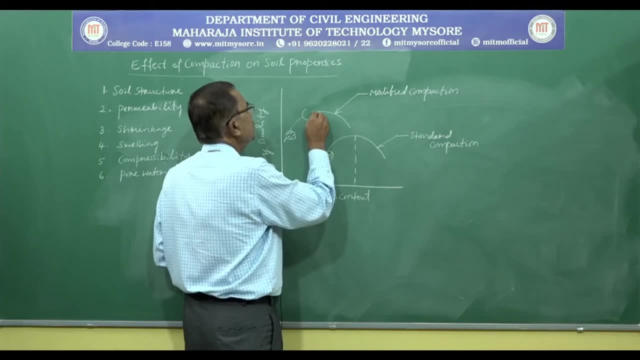 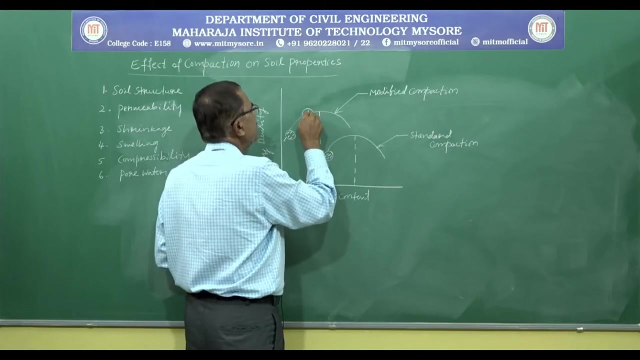 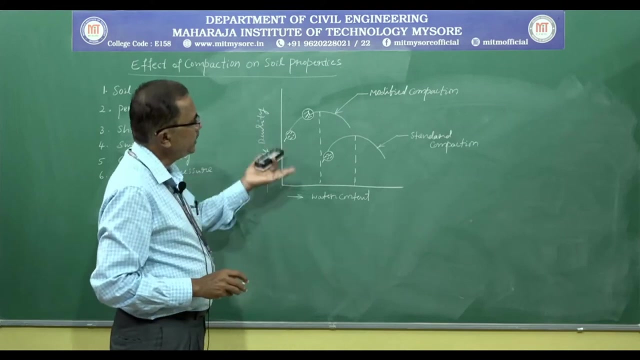 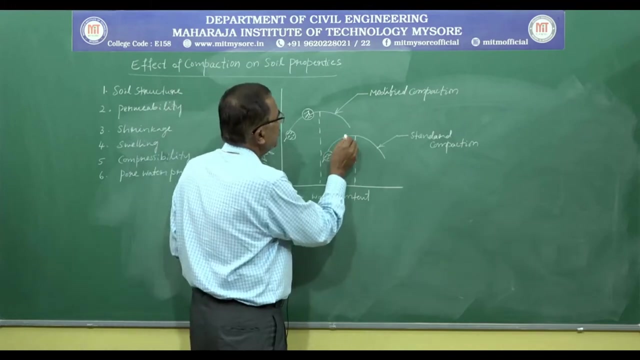 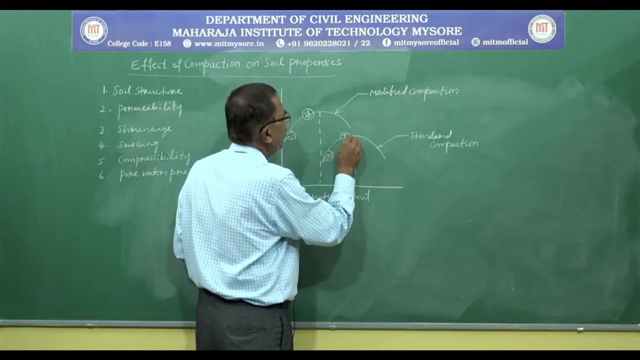 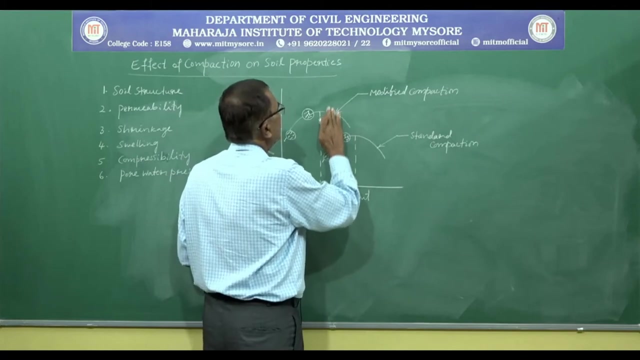 As the compactive energy increases, the edge to edge or face to face will be converted into edge to edge or face to edge to face or face to face Face to edge like this. Further increase in moisture content will alter the orientation, like this: 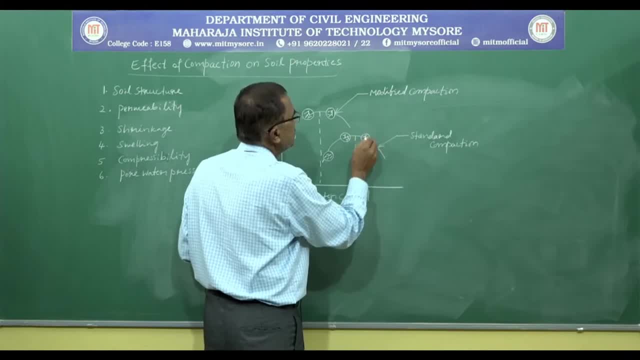 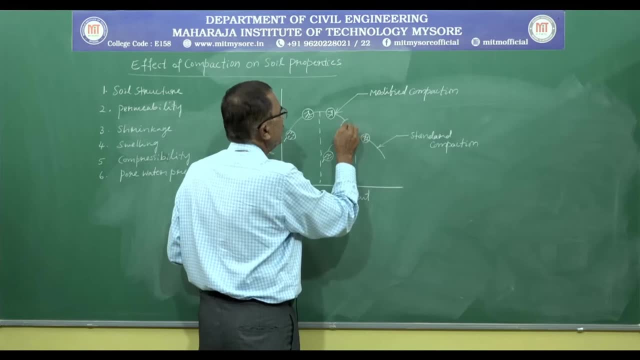 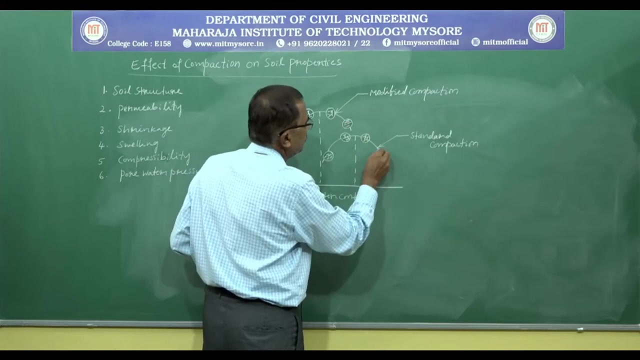 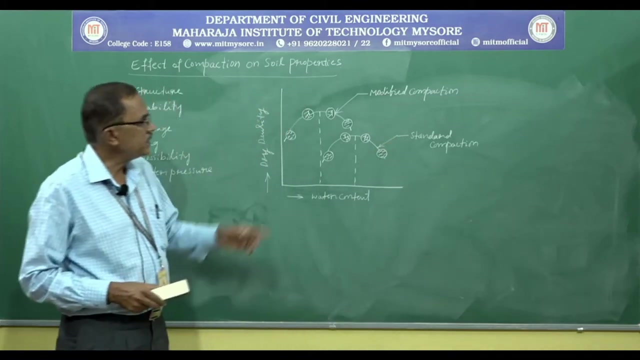 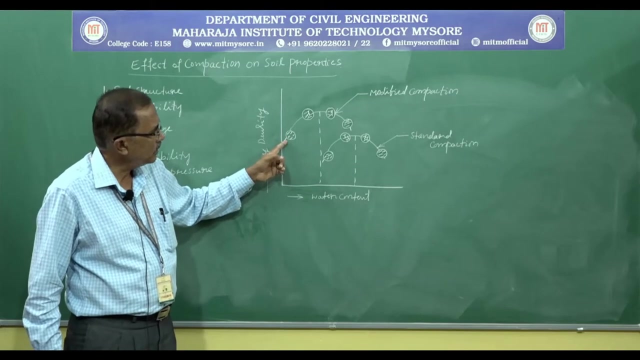 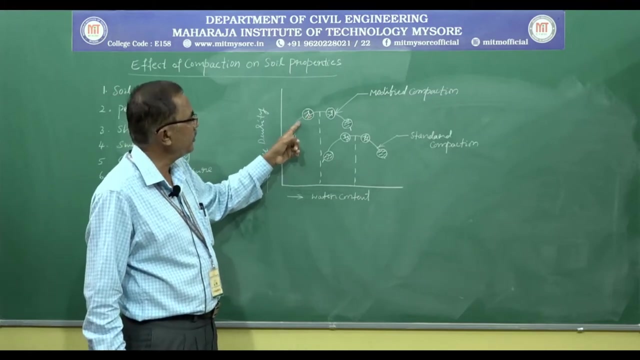 This will take place in case of addition of water content, even with the addition of with the increase in compactive effort. You can easily see here the oriented soil structures. to begin with, soils are there in dispersed structure. increase in moisture content and increased compactive effort leads. 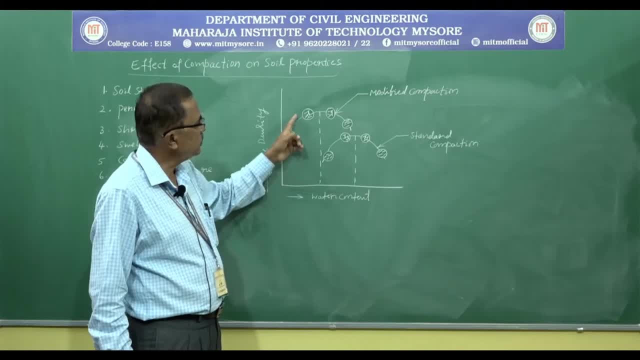 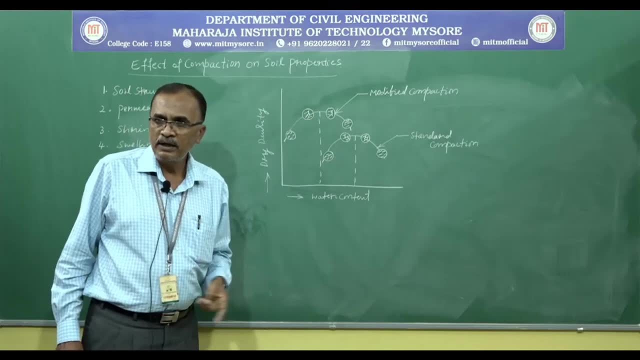 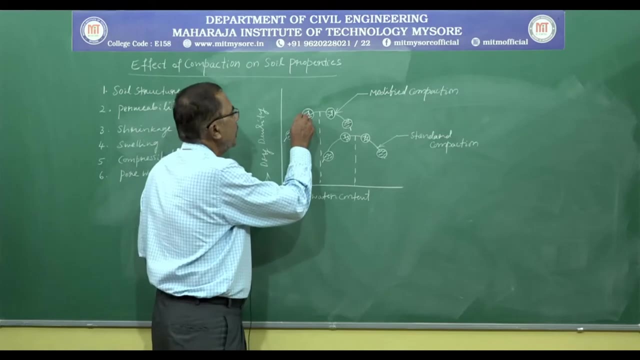 to face to face or edge to edge, into the face to edge or edge to face orientation, leading to the flocculant structure. So this flocculant structure, This structure continues up to certain limit, that certain limit also we know there is optimum. 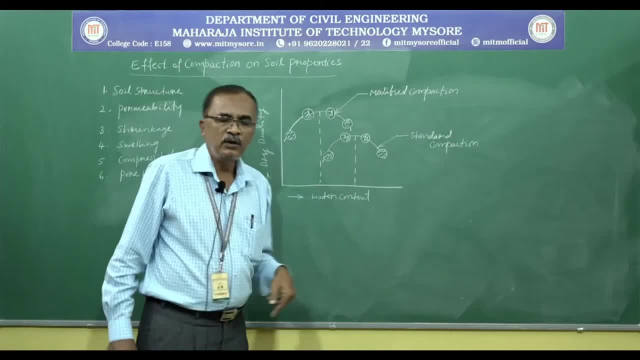 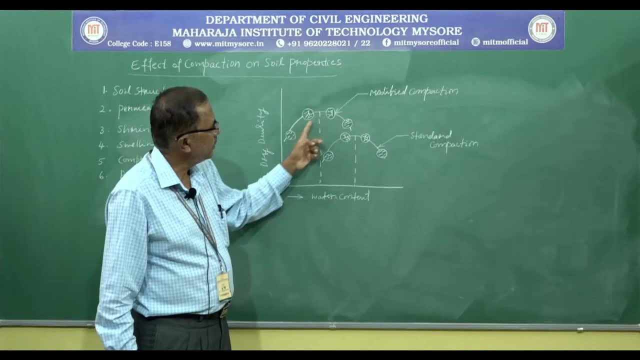 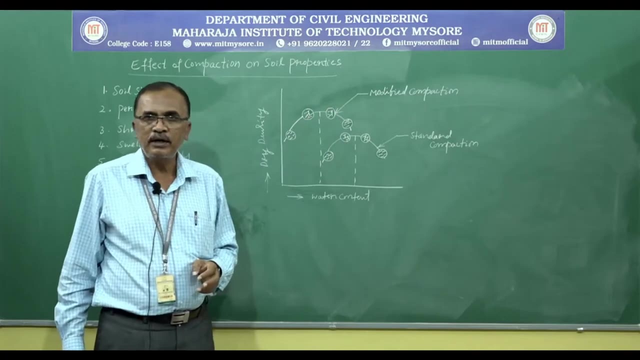 value After optimum value, with the increasing moisture content, again that edge to face structure, trying to become the face to face edge to edge. finally, further increase in moisture content leads toתhe non concentrated once dry. Is it clear The structure, The one with the top to mid edge phase or the edge to edge? so the cupl legit form hadn't? 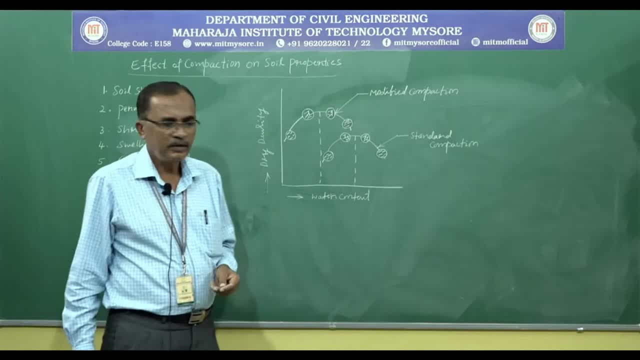 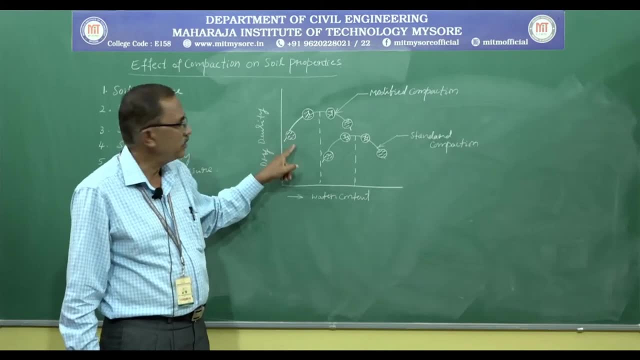 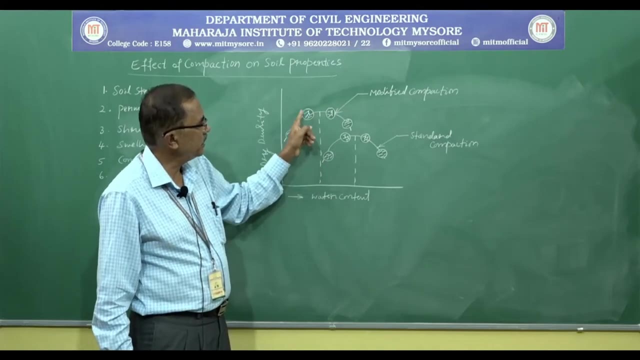 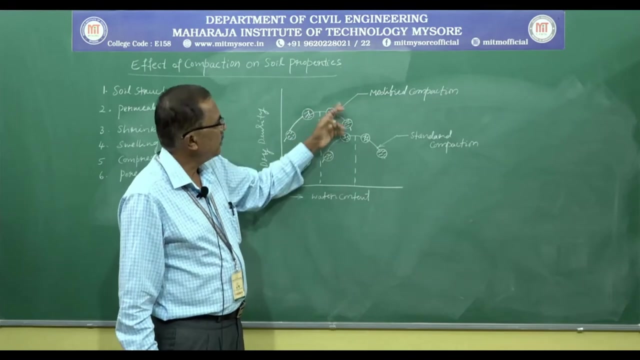 face to face or edge to edge orientation. In other words, to begin with soils are there in the disperse structure. with the increase in moisture content and compact effort, the this becomes a flocculent structure. then further increase in moisture content and compact effort after optimum value will start orienting again. then, when finally further increase in moisture. 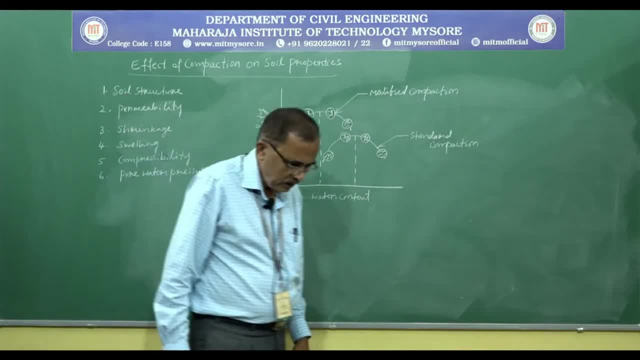 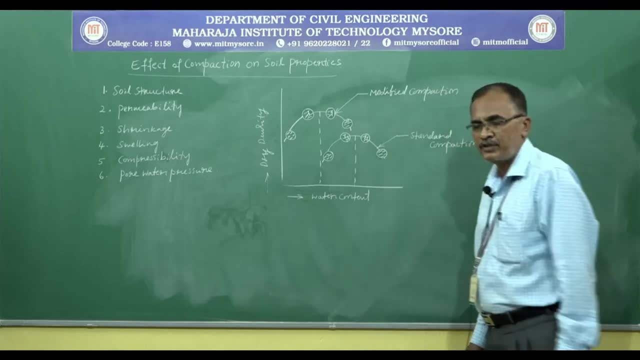 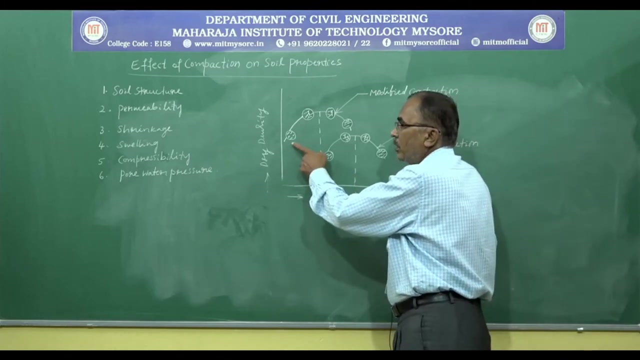 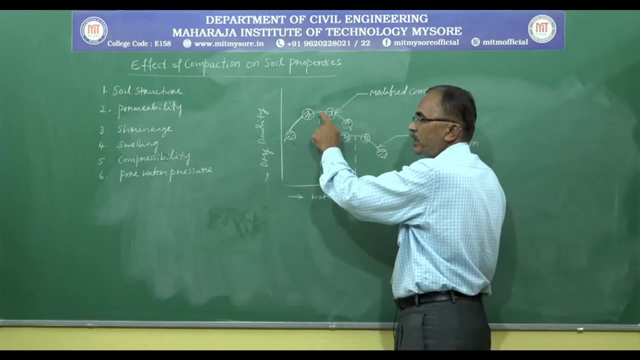 content. compact effort leads to the disperse structure. The same case is in case of standard product compaction test. So this shows that we can compact the soil to their maximum density with optimum moisture content up to certain level with the increase in moisture content. 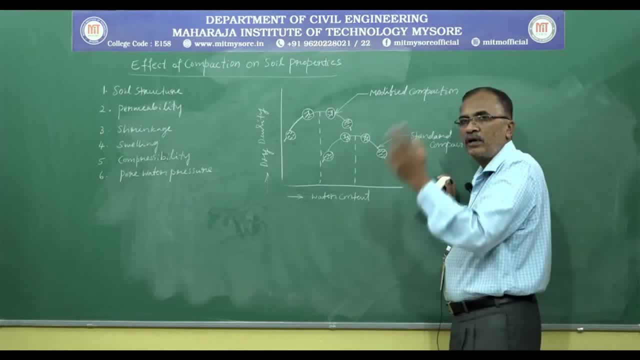 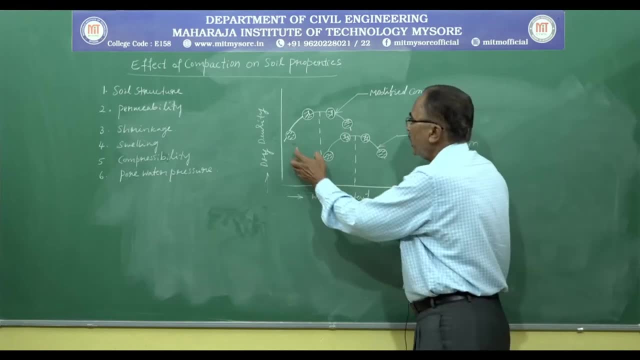 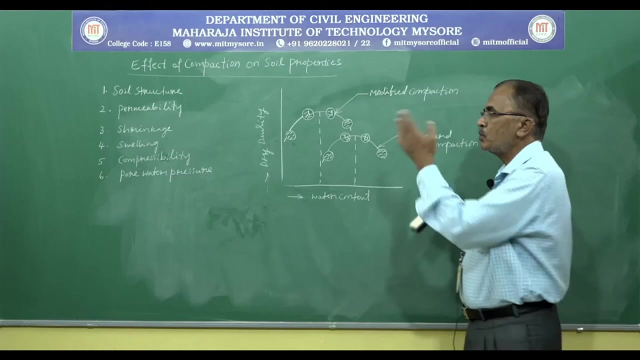 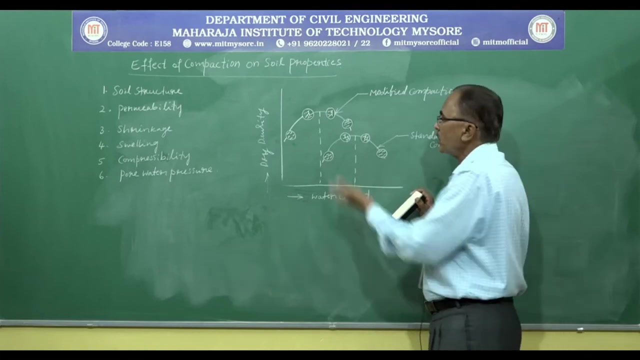 and compact effort. flocculent structure will become disperse structure. means there is a change in the orientation of soil structure or soil fabric from disperse to flocculent. up to certain level mean, up to optimum level. beyond that it is again the orientation changes to disperse structure. 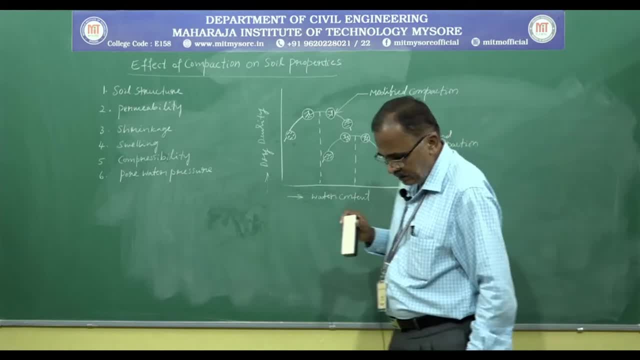 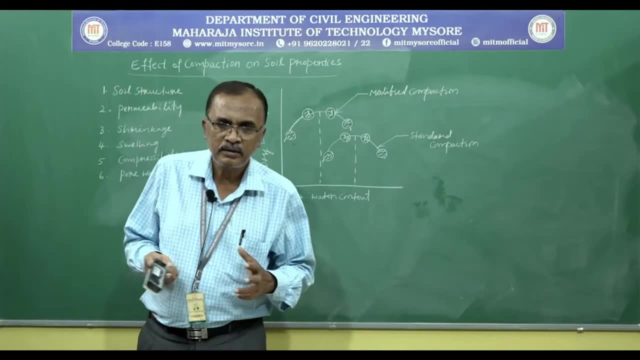 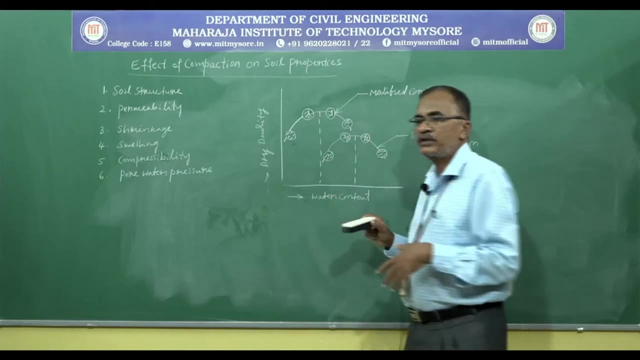 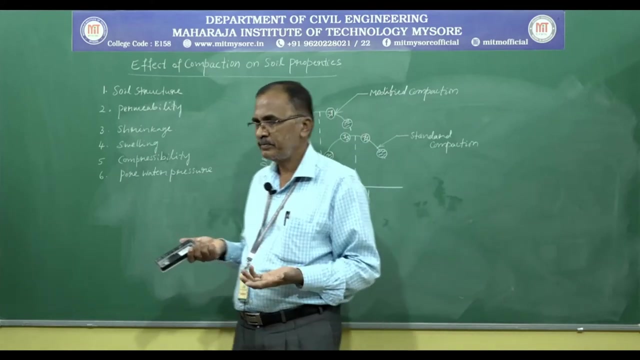 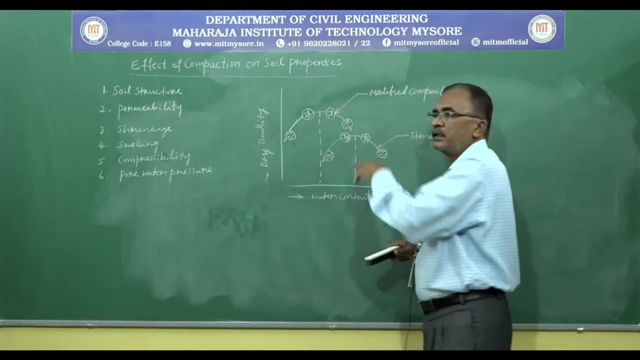 In turn. we know that already flocculent structures, though they are lighting, weight more wide ratio possess good. strength means possess very good engineering properties. the other hand, dispersed structures will not possess good engineering property. they are because of defágile towards the water. Like this, we can understand the effect of compaction on soil structure. In turn, the 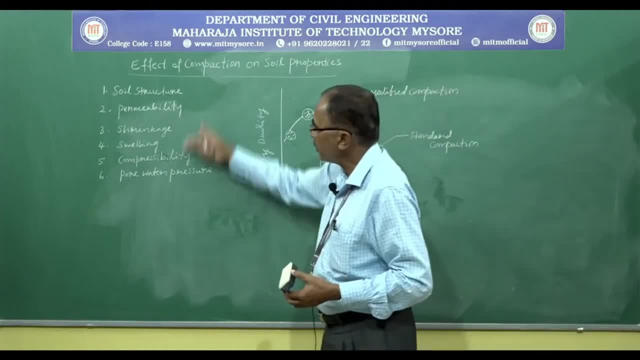 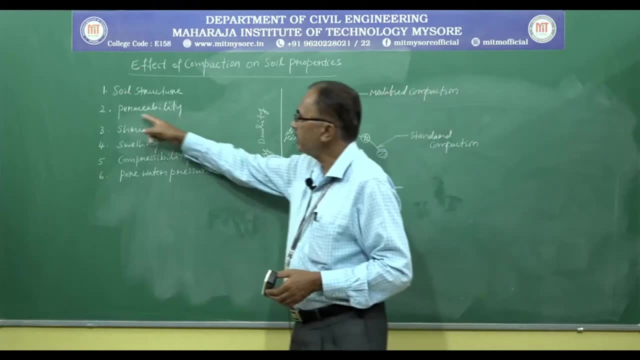 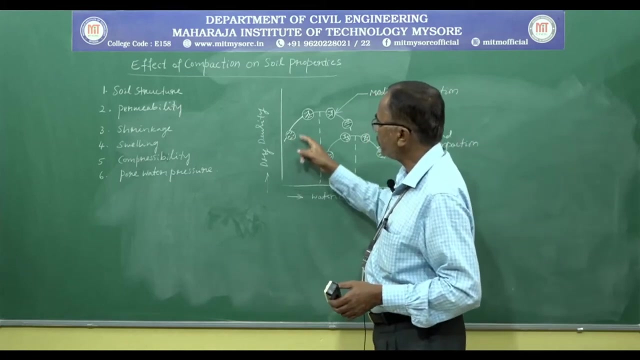 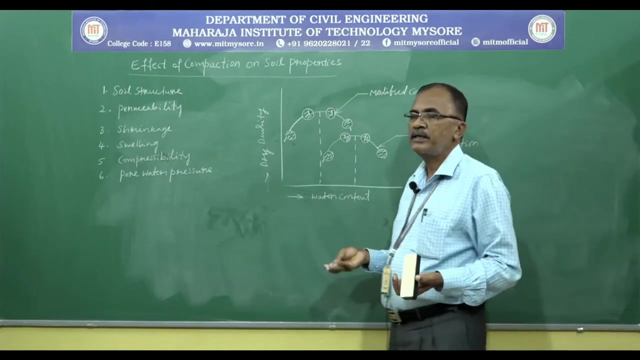 soil strength. Other properties can also be understand by using the same the dry density- water content relation. The second property is the permeability. Under dispersed condition it is, permeability is there, or some in case of coarse ground soil, and permeability will not there in dispersed structure. 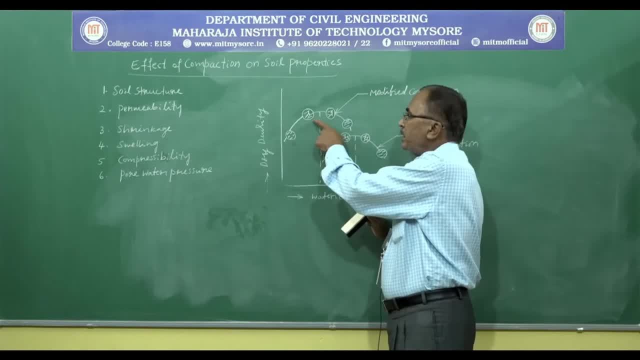 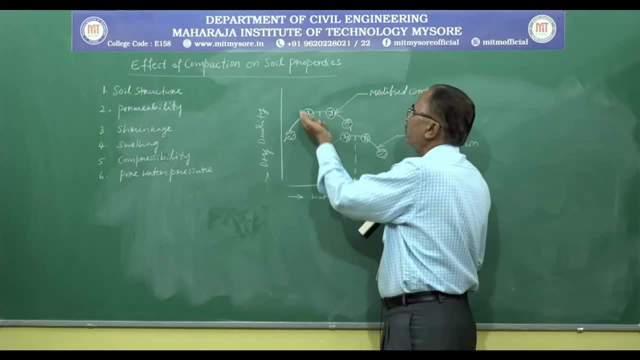 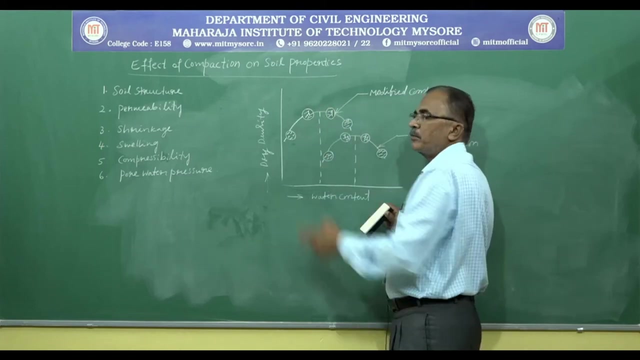 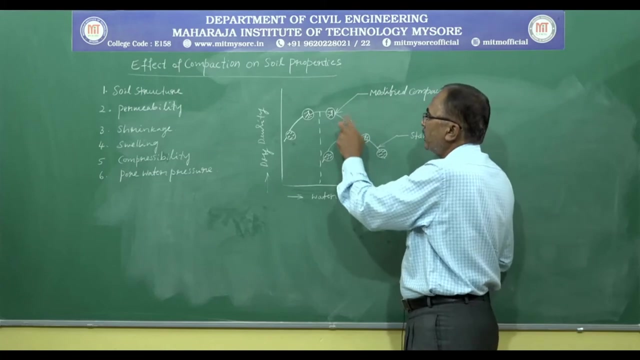 With the increase in compactive effort and water content there will be reduction in the permeability or decrease in the permeability, And further increase in water content and compactive effort leads to small increase in the permeability, And then further increase in the water content and compactive effort leads to decrease in the permeability. 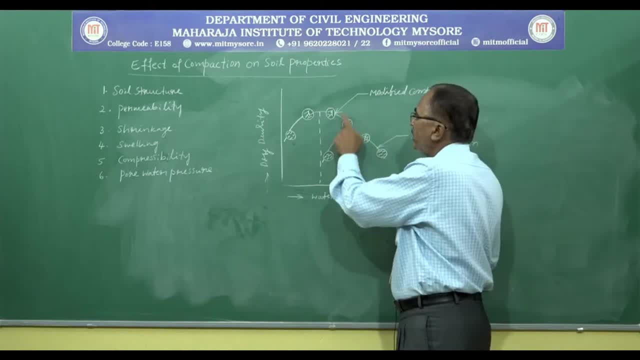 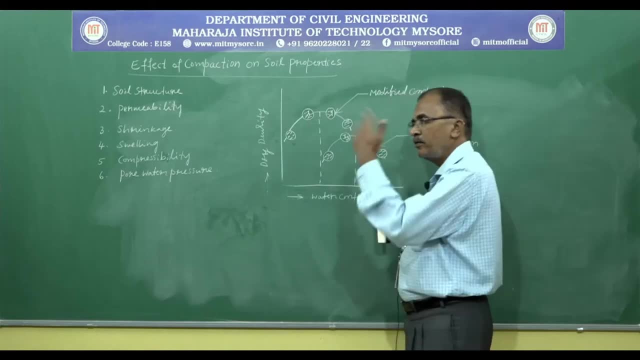 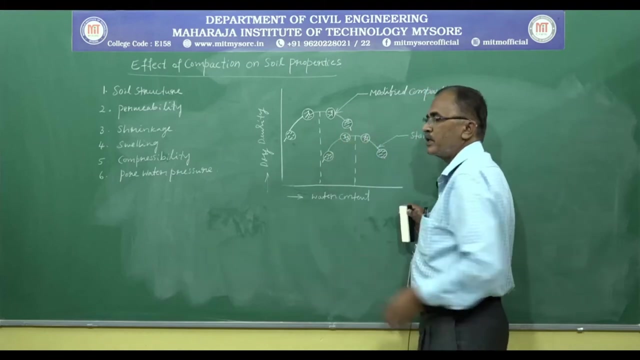 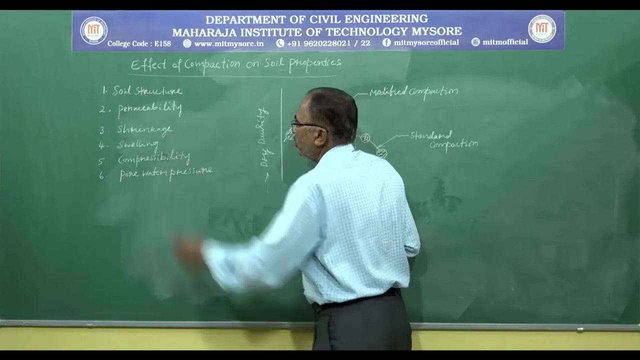 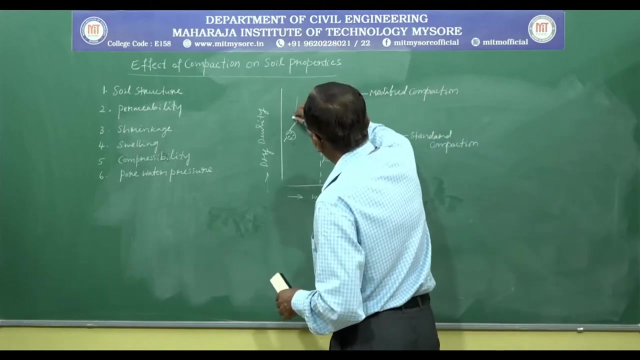 This is biodegradable because oriented, dispersed structure- Dispersed structures of soil will not leave water easily, even with mechanical effort, extra mechanical effort. The same is the case in standard compaction test, also Coming to this third property- shrinkage, compacted soil can be grouped into like this: 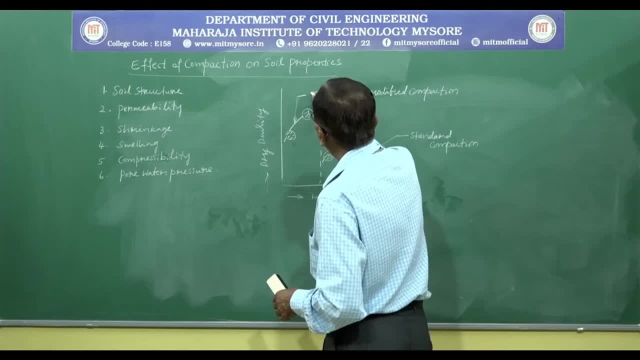 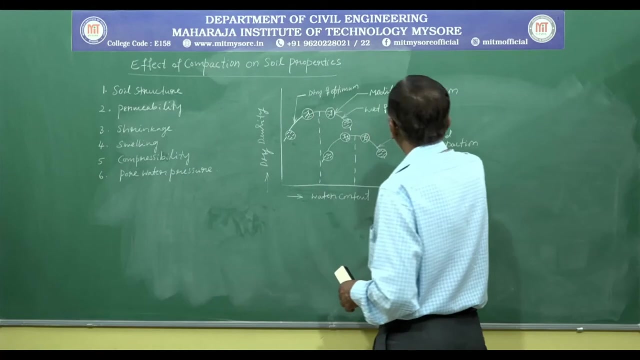 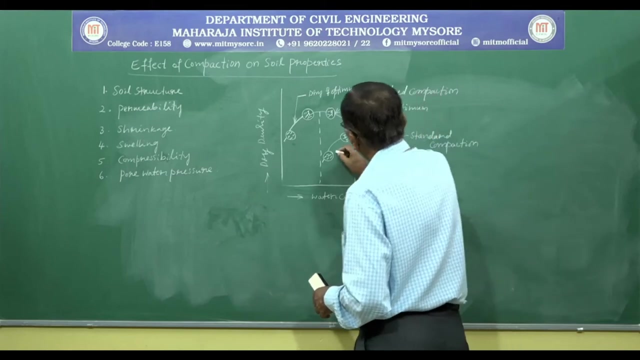 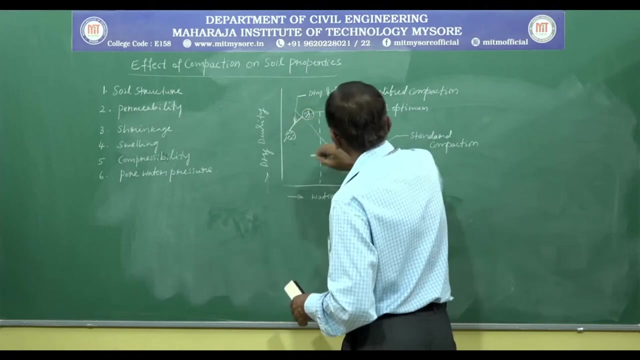 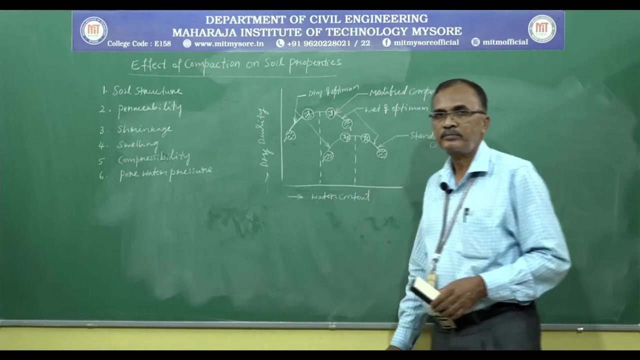 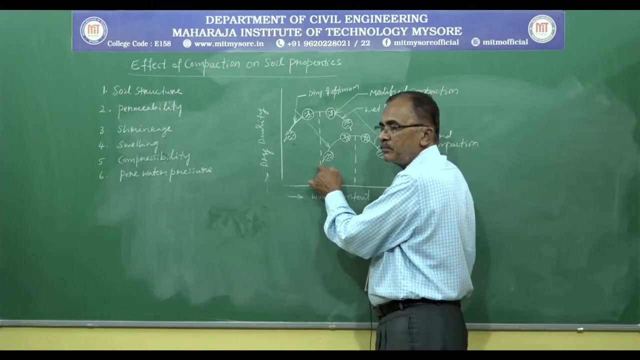 It is based on compaction curve. This is dry of optimum and this side we call it as compacted Wet of optimum. So again, here also it is. this is dry of optimum and wet of optimum. Soil compacted: dry of optimum. Soil compacted: dry of optimum. 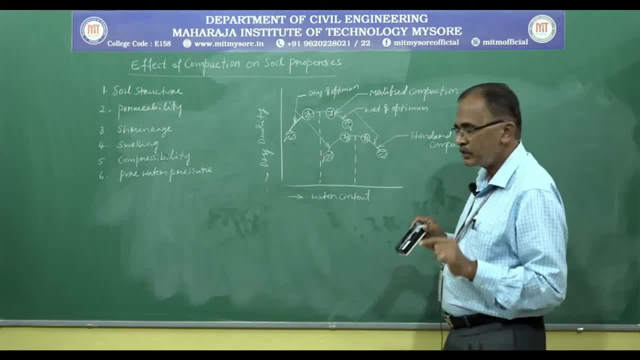 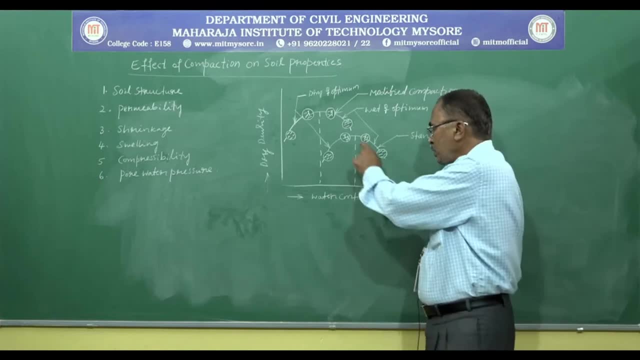 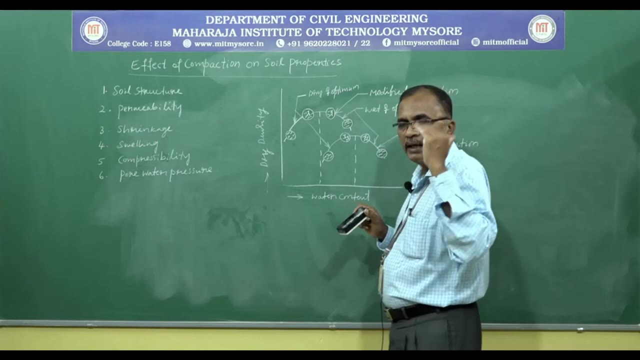 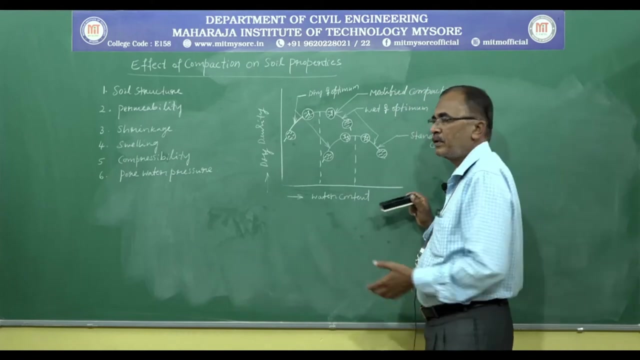 Soil, compacted, dry of optimum, will possess voids, possess both water, to a smaller extent, and air. When they reach to the optimum level, there is reduction, comfortable reduction in air voids and with optimum value of water context. So this, the dry condition of the soil, will have the affinity towards. absorbing water and upon application of load, there is less reduction in the volume. As a result. shrinkage is less if soil compacted dry of optimum and it is more the soil compacted in with wet of optimum. So these cases are more predominant in case of fine grind soil than coarse. 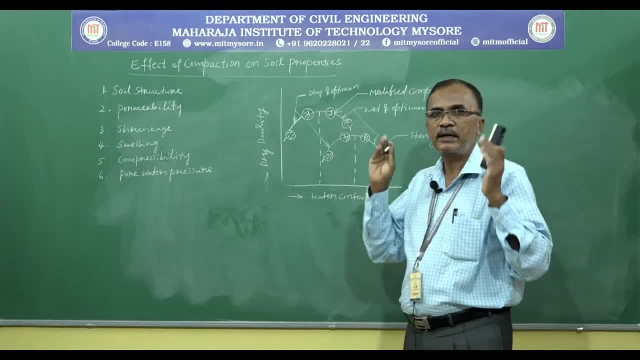 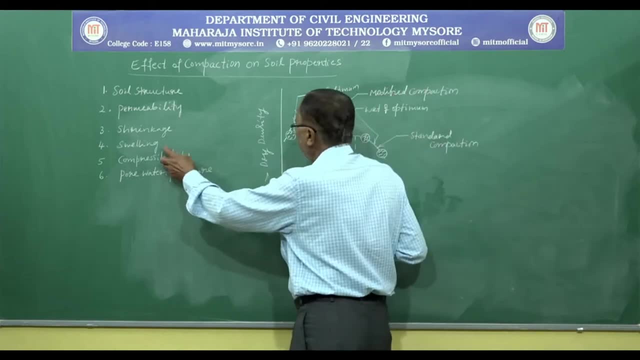 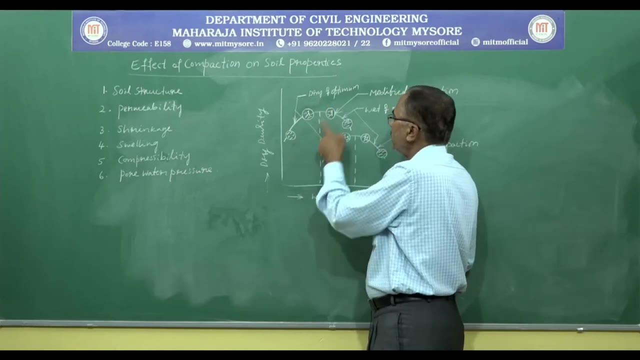 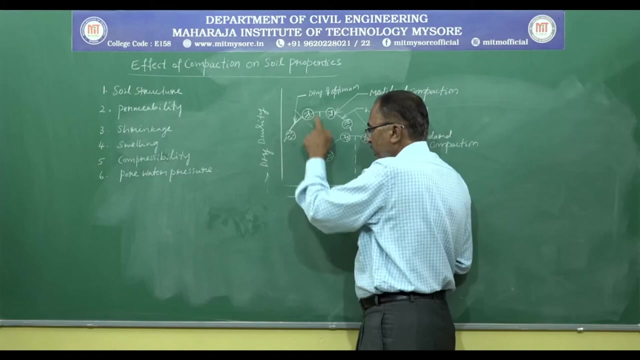 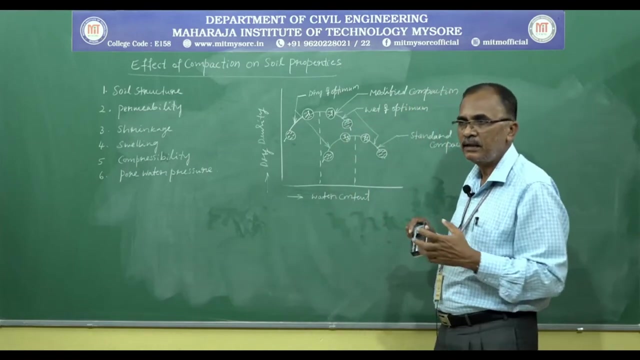 grind soil, as coarse grind soils are having less affinity towards water. Coming to fourth property: swelling: soil compacted dry of optimum having more swelling than the soil compacted wet of optimum. Here, less water contained during dry compaction leads to absorption of water. As a result, clayey. 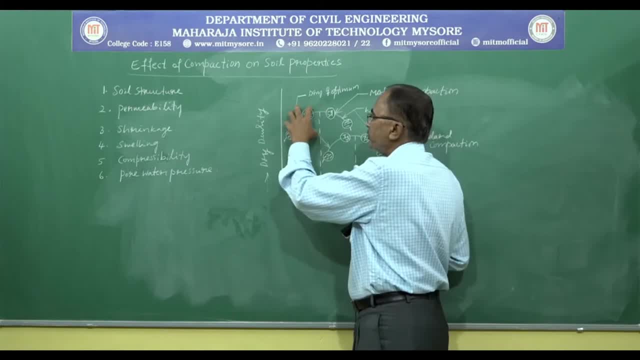 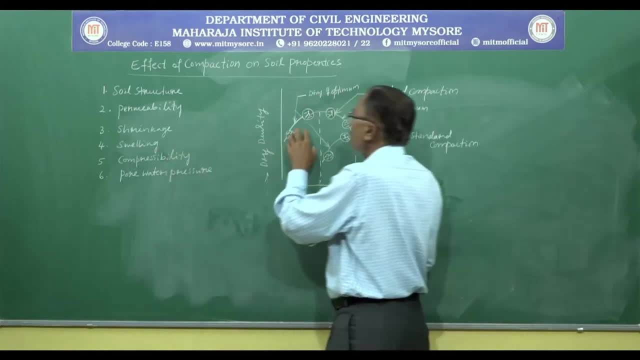 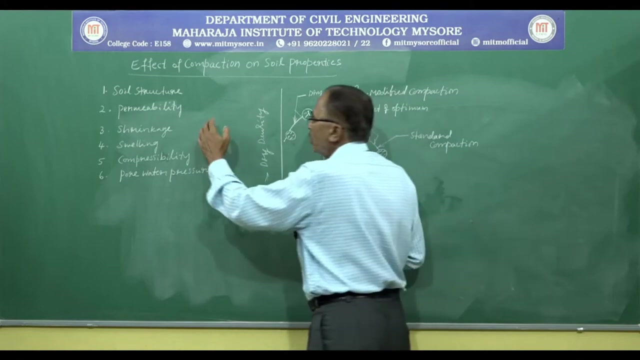 soil swells under a dry condition and the same is not in case of wet of optimum. In other words, swelling is more in the clayey soil compacted- the dry of optimum- than wet of optimum, and shrinkage is minor In case of fine grinding soil compacted, dry of optimum. Here, less water contained during. 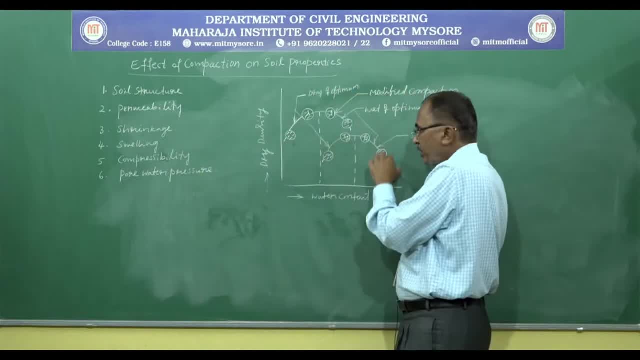 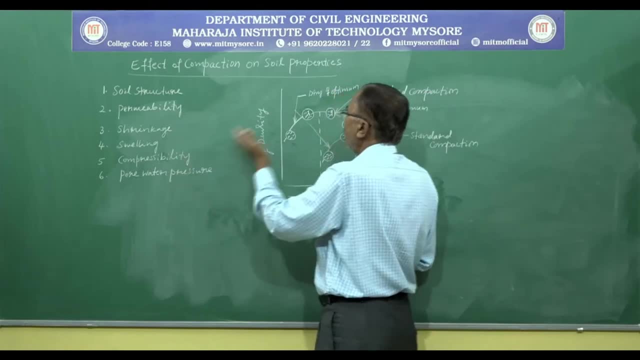 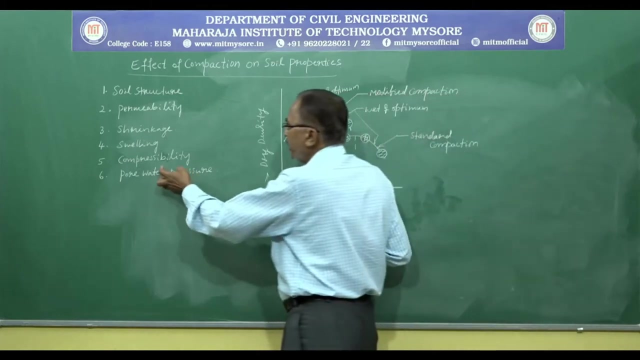 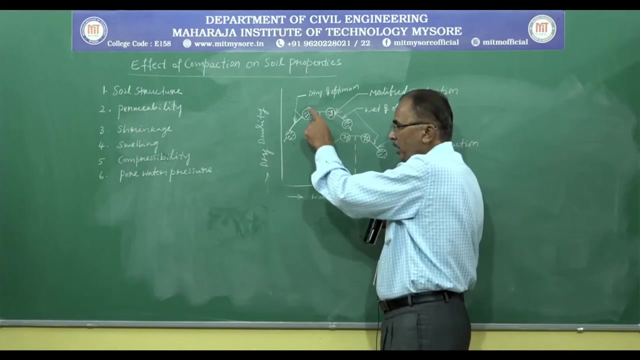 more when soil compacted, wet of optimum than dry of optimum. and for this swelling and shrinkage, again we can correlate with the soil structures: Compressibility, here again, soil compacted, dry of optimum, having a flocculant structure and this flocculant soil with flocculant structure will 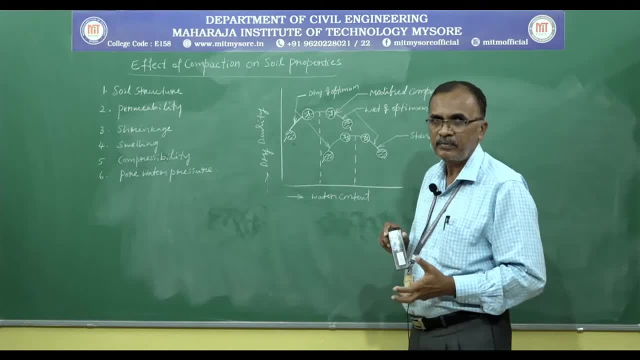 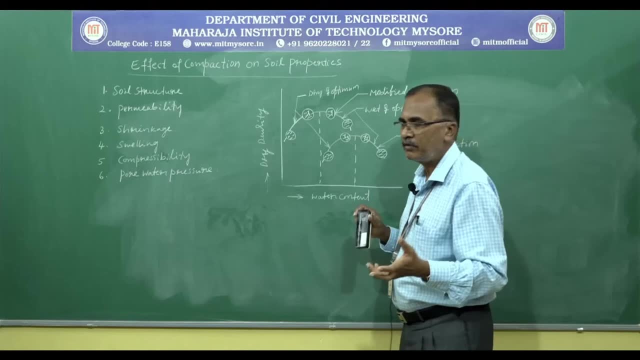 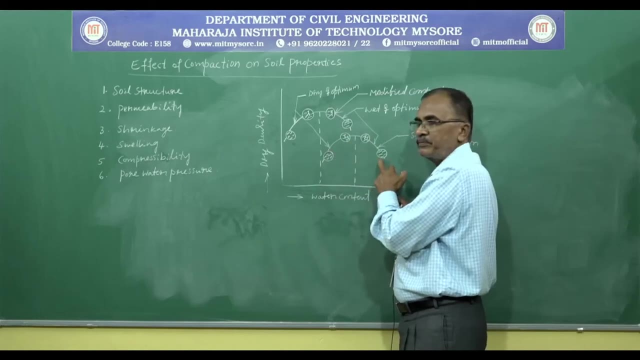 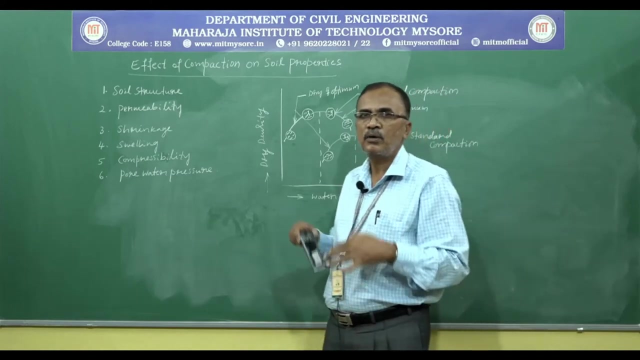 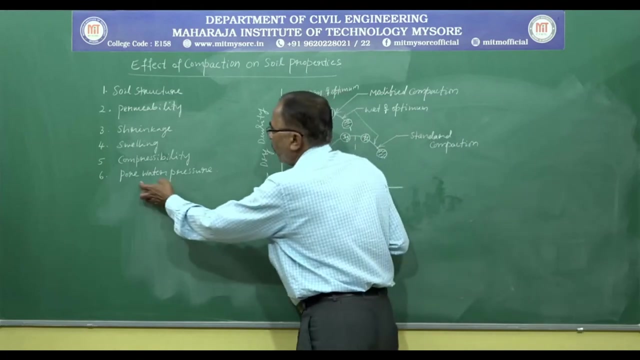 resist load effectively, Whereas soil compacted, wet of optimum, will not resist load effectively. as a result, there is more settlement means there is more compressibility of soil, So dispersed structures in soil lead to more settlement. Lastly, pour water pressure. pour water pressure means particles. the gap between 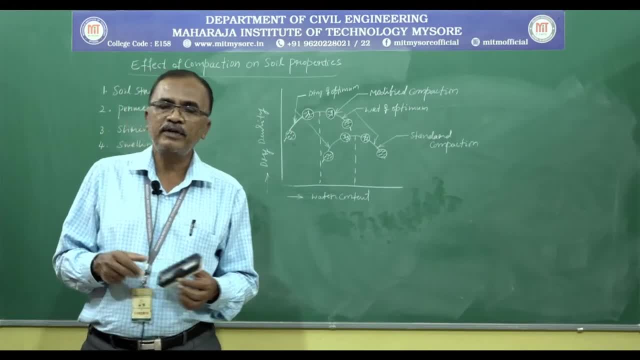 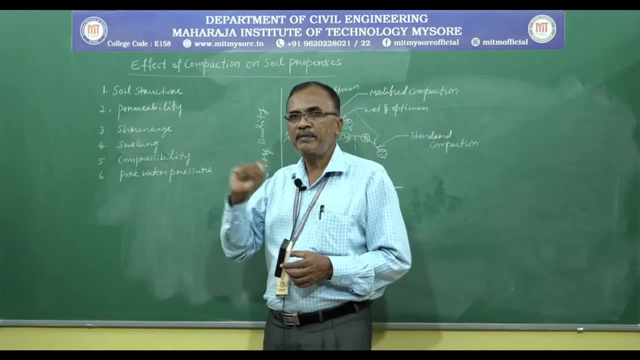 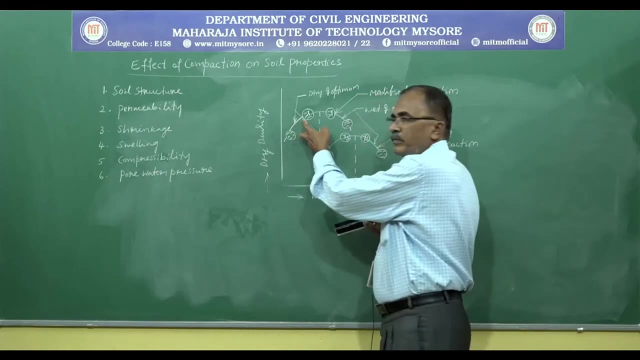 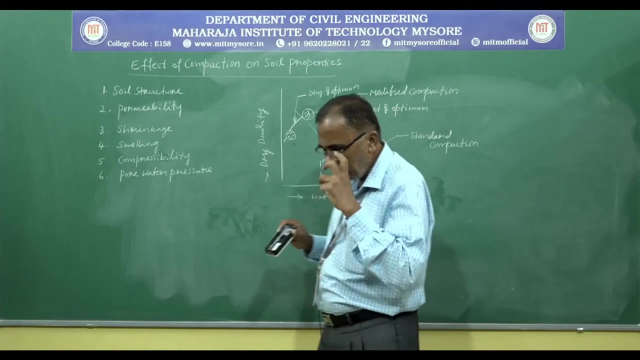 the particles are called as pour. For our convenience we use that gap as void. Pour means gap between the particles is known as pour. In that gap when we keep on adding more water here it is soil compacted. dry of optimum will lubricate the soil particle and facilitate. 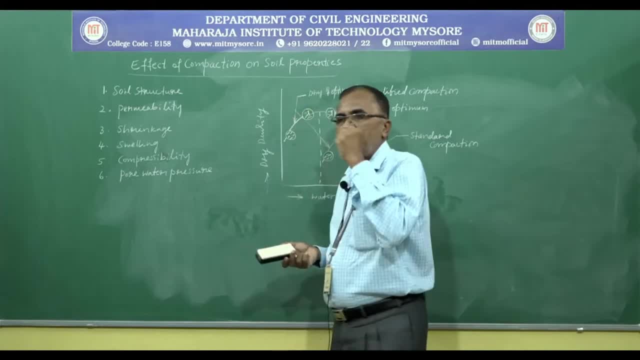 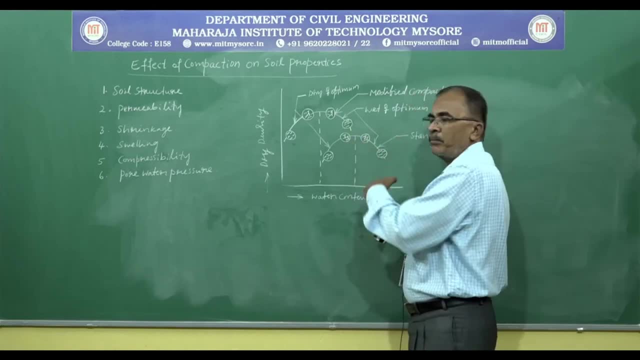 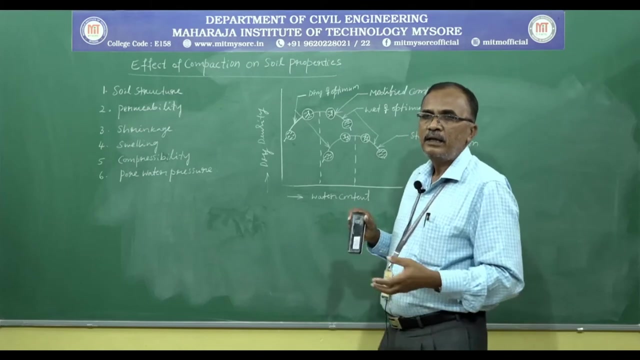 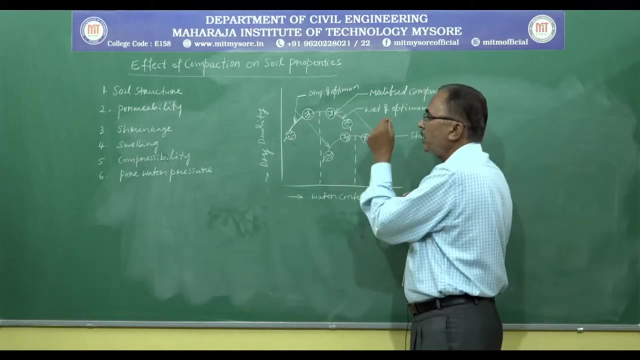 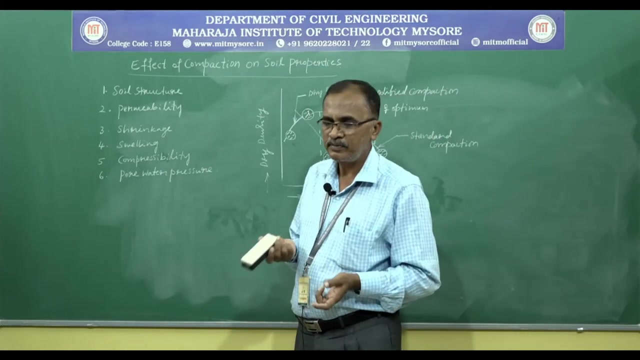 for easy movement of the particles. hence we can increase the density. On the other hand, if we compact soil beyond optimum point or optimum level, increased water content leads to replacement of voids by water. These replaced water will held within the soil and that water will exert pressure on soil particles. When water will exert pressure on soil particle. 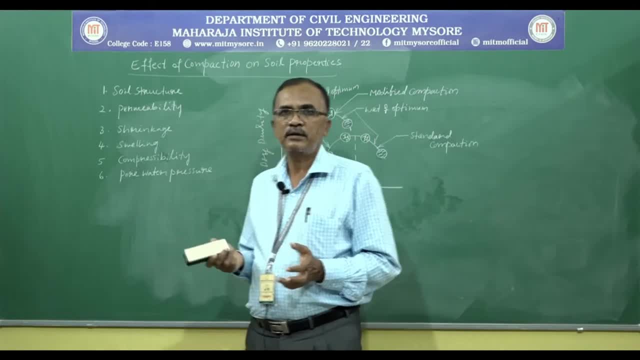 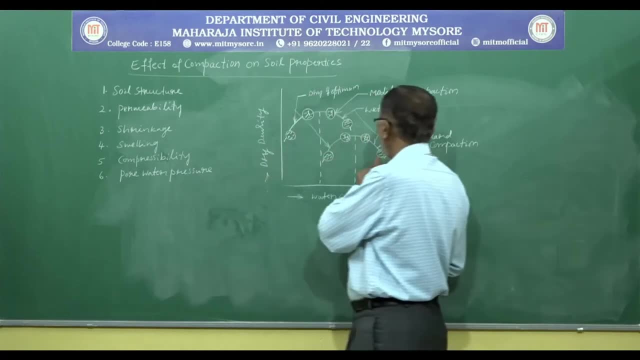 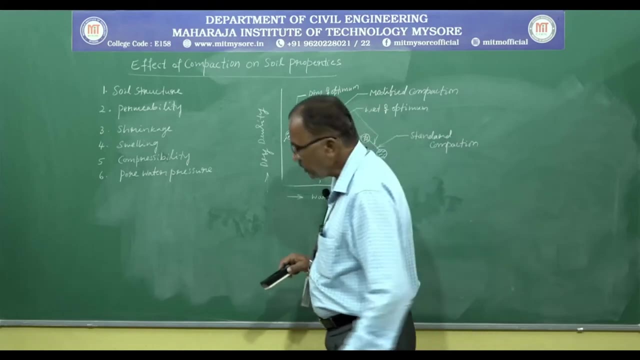 it will try to reduce the density in turn, all engineering property. So pore void pressure is the density of the soil, So pore void pressure is the density of the soil, So pore void pressure is more, in case of soil compacted, wet of optimum than a dry of optimum. So these are all the 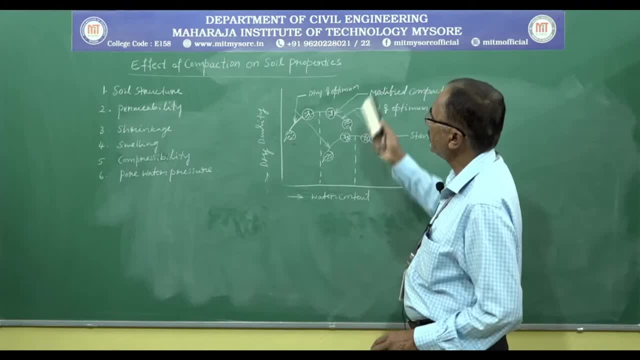 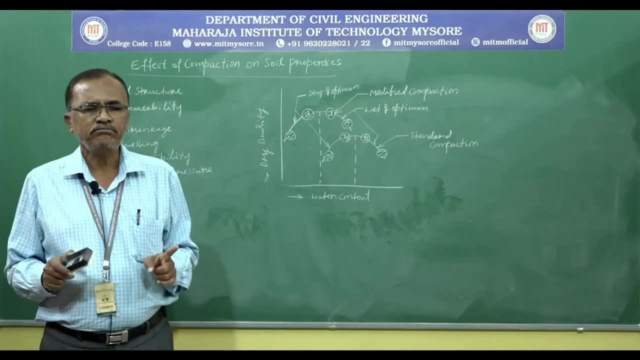 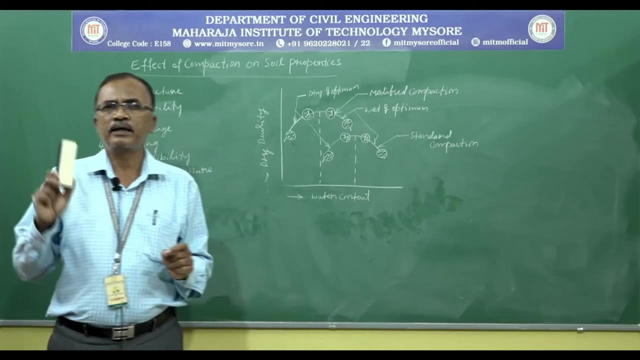 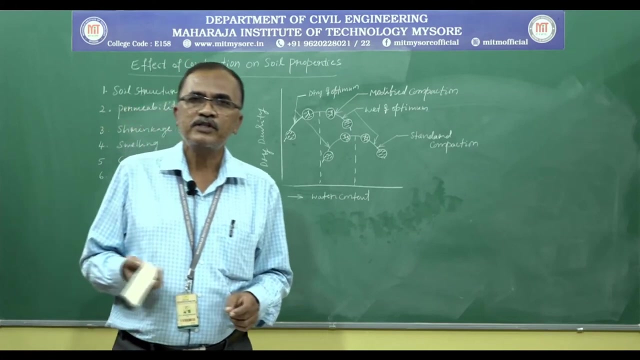 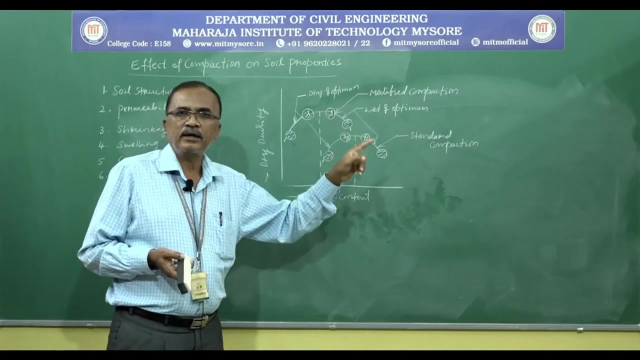 effect of compaction on soil property. that is what we mentioned there in differentiating between compaction and consolidation. So compaction is a simple phenomena and consolidation is a complex. sorry, compaction is a complex phenomena and consolidation is a simple phenomena. complex phenomena means do. while carrying out the compaction, we should take care, and there is a control here under 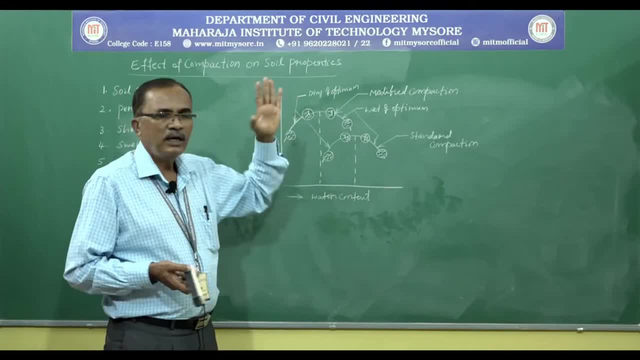 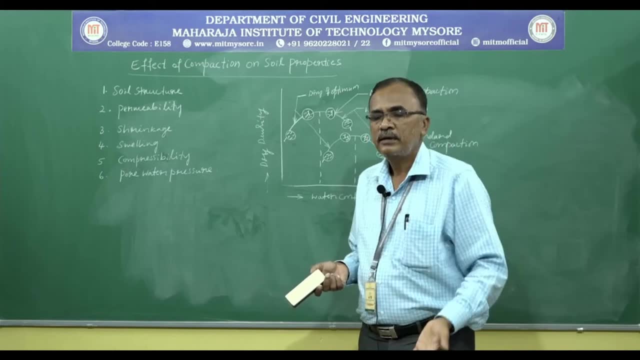 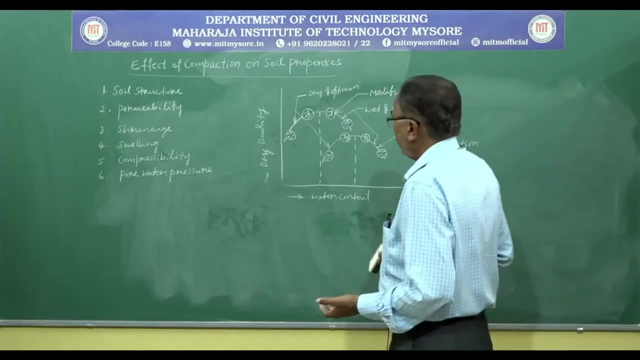 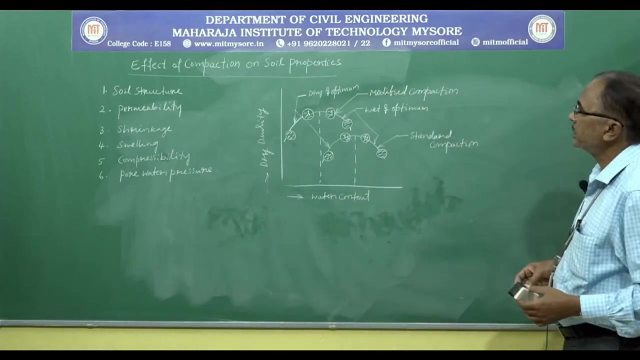 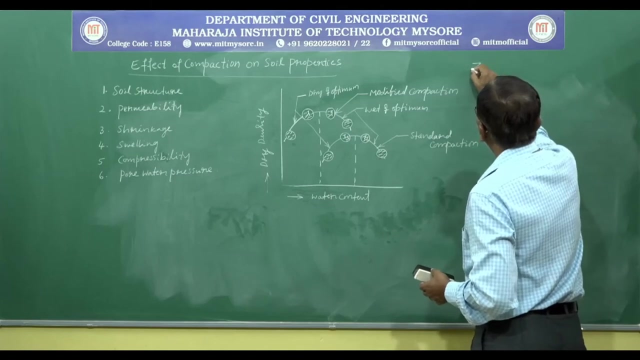 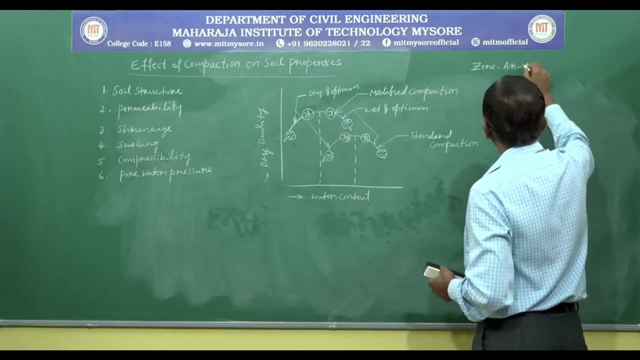 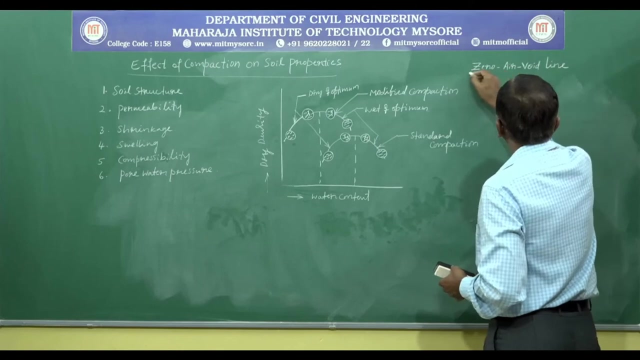 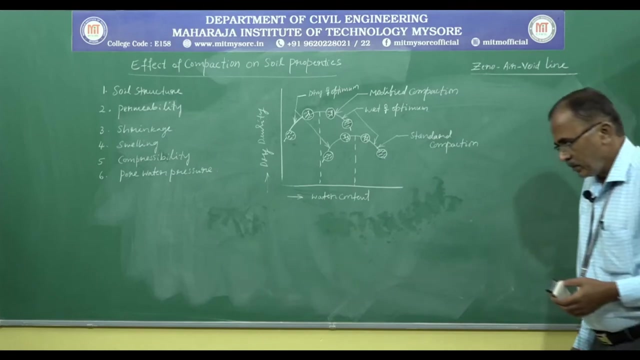 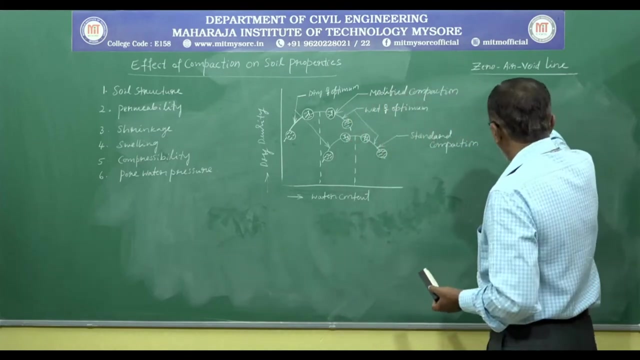 controlled condition. we do compaction to achieve the desired density under under the optimum moisture content and compact you effort. then, after studying this effect of compaction and soil property, let us consider another interesting topic. it is called as zero air void line. so from the compaction test we can establish the relationship between dry density and water. 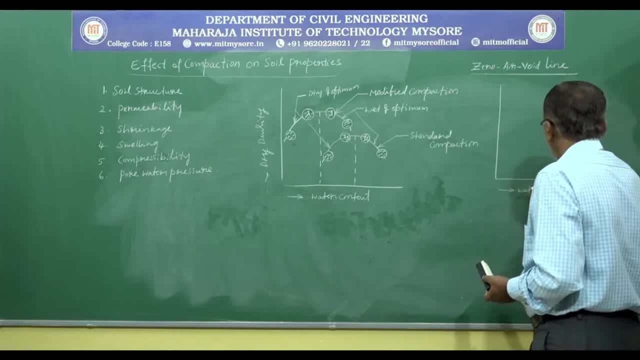 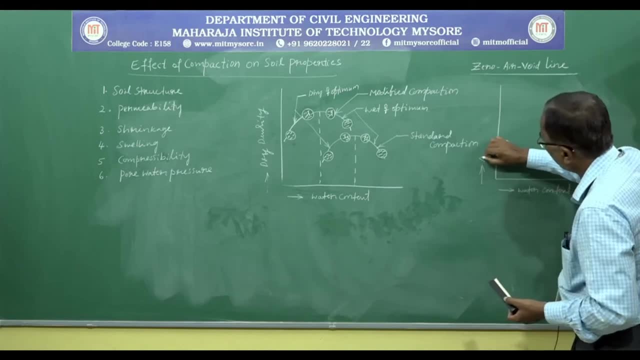 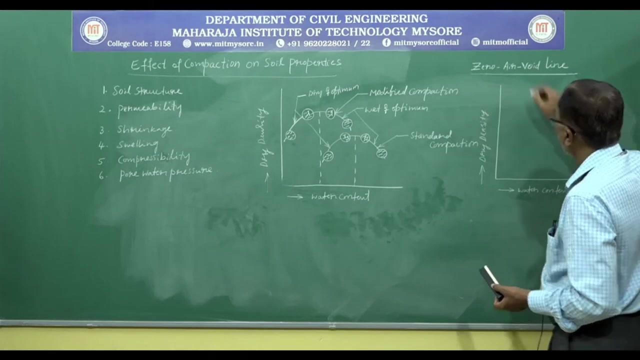 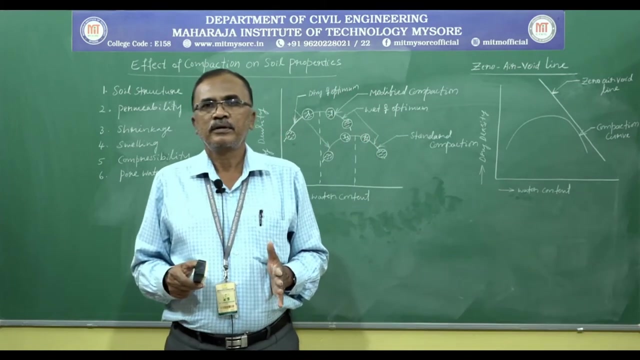 content and this is the compaction curve. we can also obtain a curve or a line tangential to the line. width of optimum compaction curve is known as zero air void line. the objective, very objective, of compaction is to reduce the air voids. reduction in void. 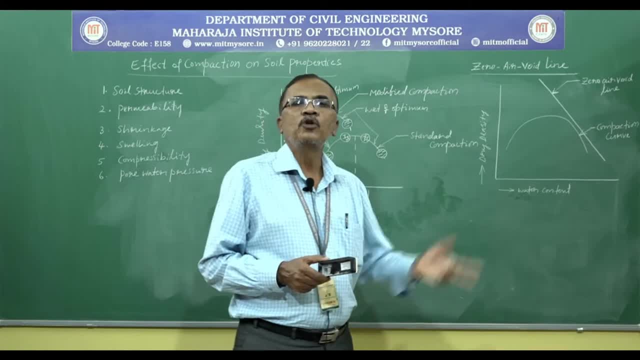 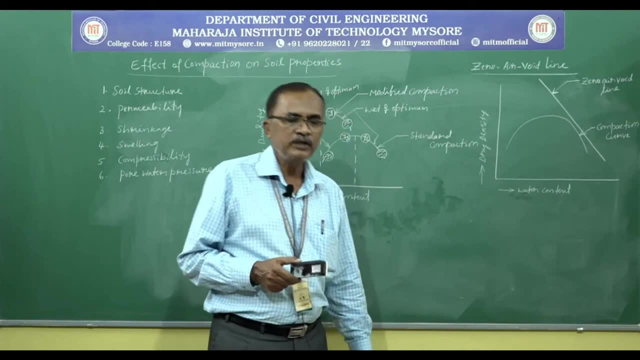 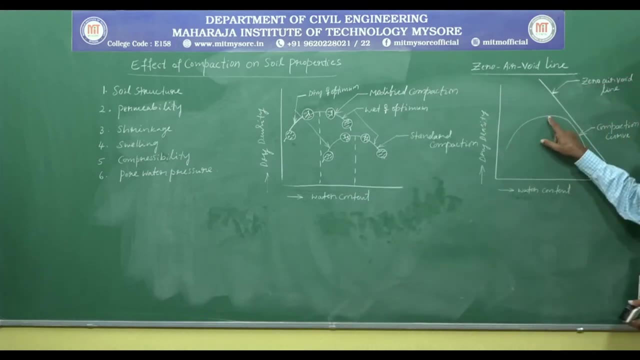 void in soil after optimum lubrication of soil particles will leads to increase in the density increase density will leads to increase in all the engineering properties. when we reach to the optimum level during compaction, it is assumed that voids are reduced to maximum extent, almost to zero. 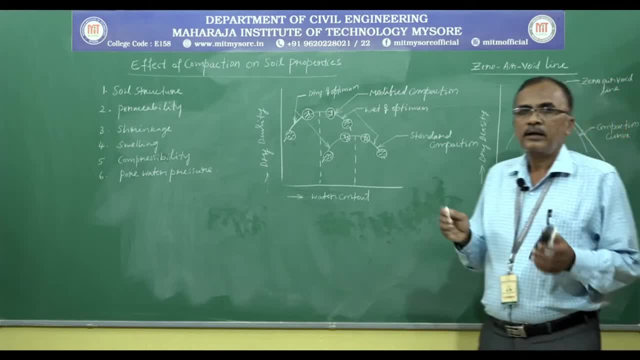 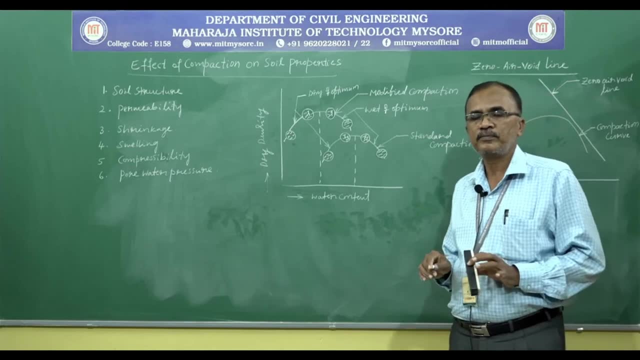 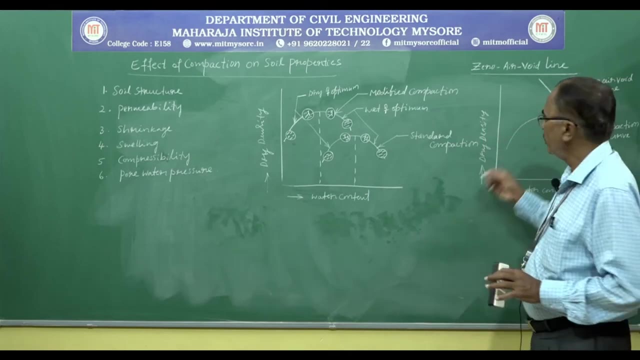 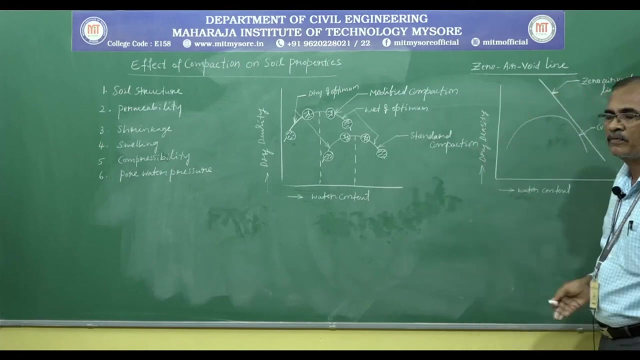 but it is not so. but reduction of voids to zero is highly impossible. it is not possible to reduce voids to zero. honestly. he's have a practical purposes. when weirid the optimal level of maximum level, we simply assume that it is to be a two-day and I was a member club will need to be at that. zero of wights is zero, zero. you'll be very sorry. one question is. 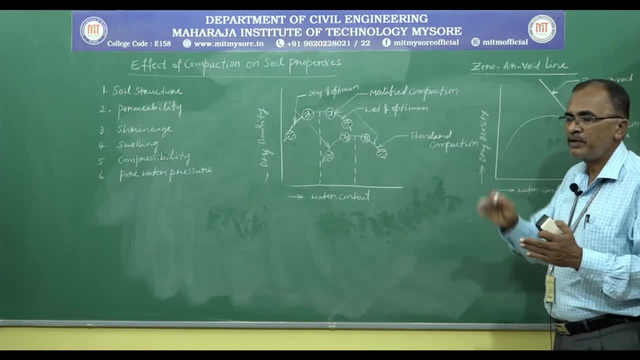 one more question is notebook. would you change a for and tea or just to write all the education to drill anyone. one function that it's just an article word here as a general, but if not more then ouvert and change one expression, then it united transfer area, still not one before this. as a flybert place to new volume rate or other place will not match like a slow pace over the fill of theiser facebook. 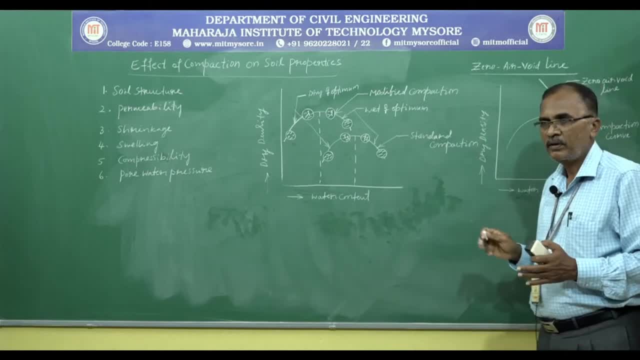 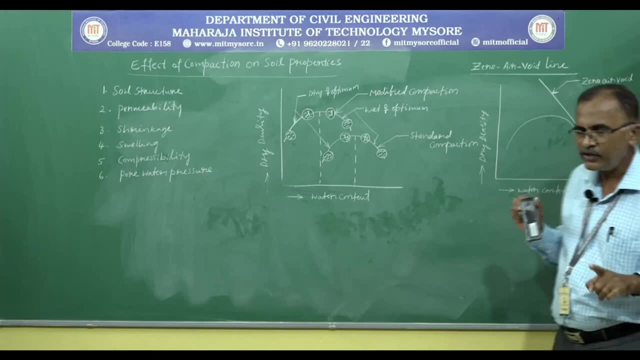 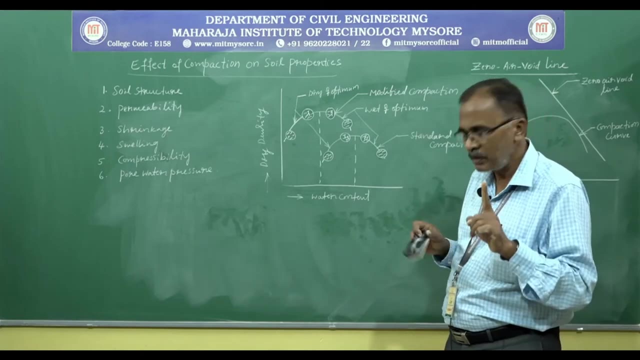 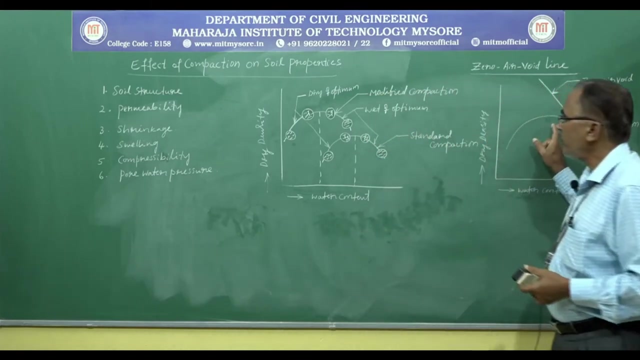 fight exam. air voids are zero. Under such circumstance it is like degree of saturation for saturated soil. we take degree of saturation as one means all the voids are completely filled by water. we take degree of saturation one Here also, we assume that all the voids are completely removed. all. 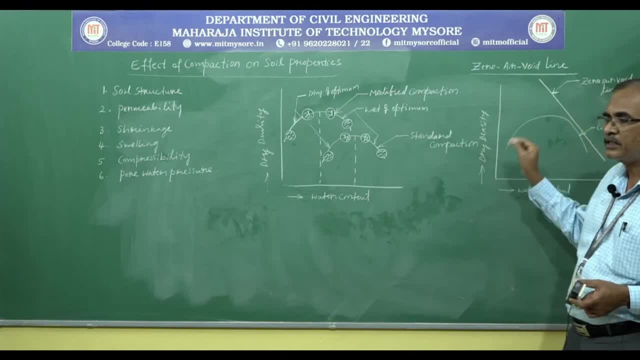 the air voids are completely removed. Hence we can consider that condition as a saturated condition for removal of air voids. Hence this zero air void line can also be called as saturation line or 100% saturation line. Zero air void line or this 100% saturation line will never cross the compaction curve. 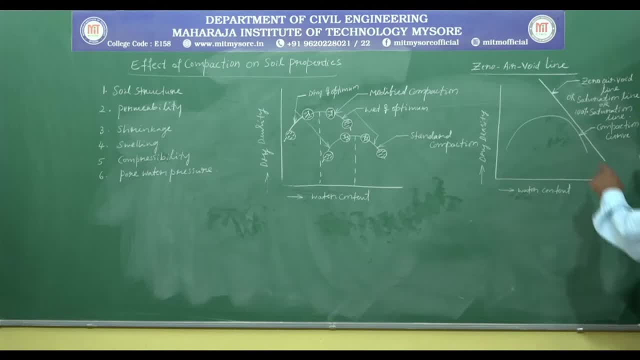 So here we draw this line by assuming that fact, assuming the fact that there is no air void in the soil. So here we draw this line by assuming that fact, assuming the fact that there is no air void in the soil. So here we draw this line by assuming the fact that there is no air void in the soil. 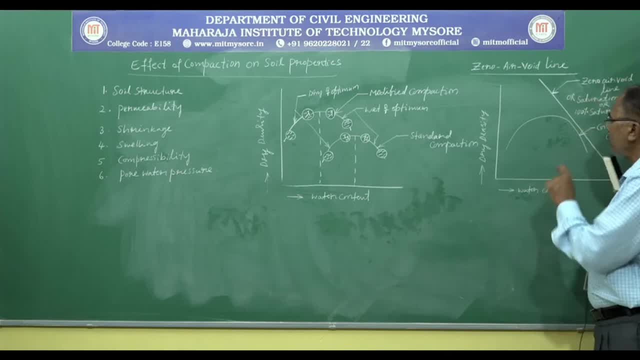 For 100% saturation. no air void means it is. degree of saturation in terms of air voids is 100%. it is one market For different wet water content. we can obtain the again the density. So density at zero air void can calculated using density corresponding to water content: zero air void, density corresponding. 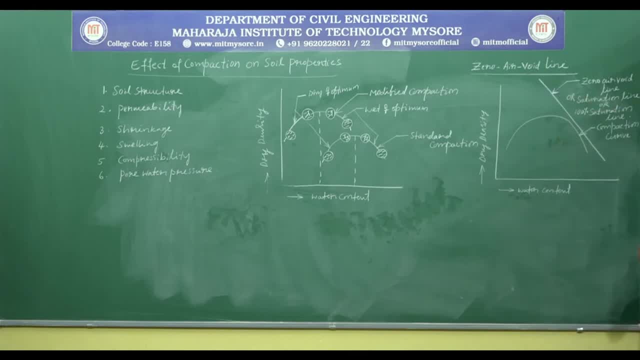 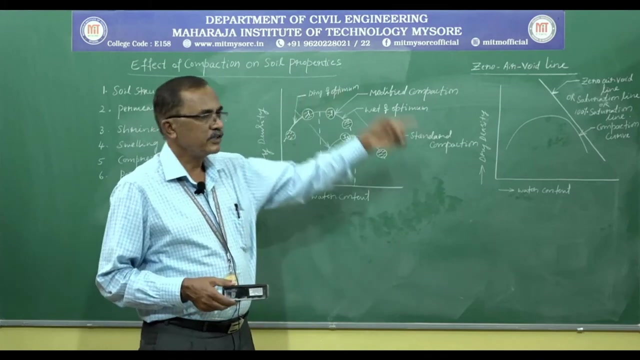 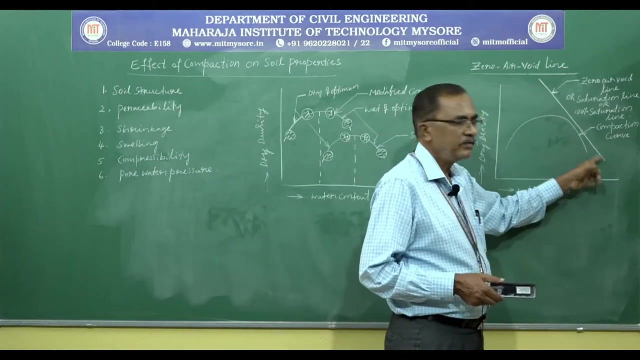 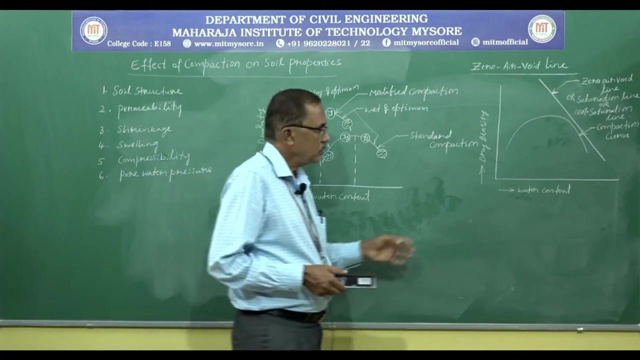 content. we can obtain this zero air void line or the saturation line, and this zero air void line or saturation line will serves as a. we can call it as a check for the accuracy, as this zero air void line or saturation line line will never cross the the compaction curve. So this is for 100 percent saturation line. we can also draw 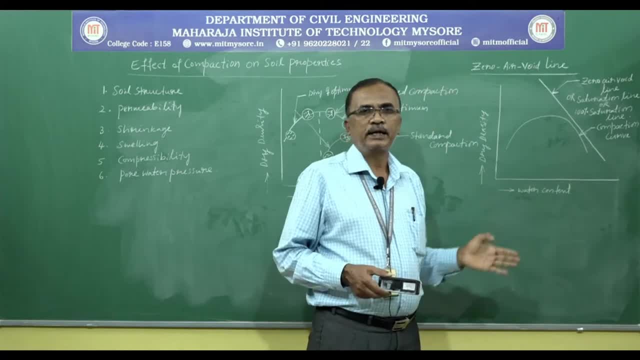 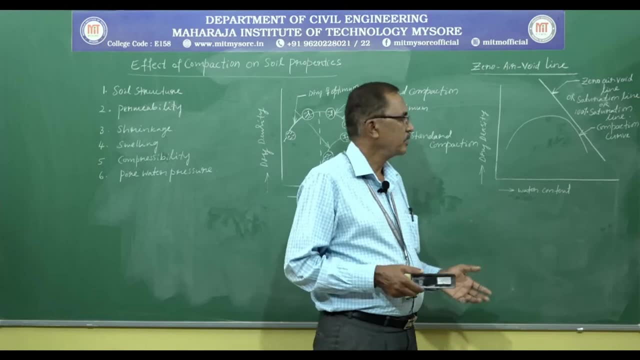 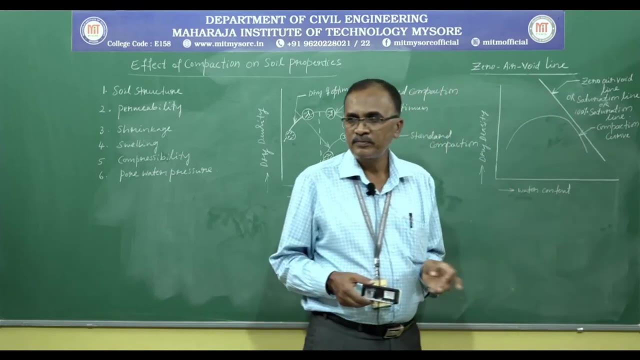 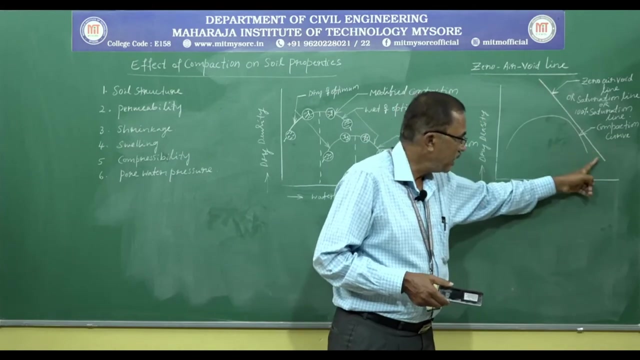 the saturation line corresponding to 80 percent, 70 percent, 20, 60 percent, like that for the desired saturation level. under that circumstance, the this the saturation line will cross the compaction curve For zero air void line. always it is this. that line is parallel to the wet of optimum compaction curve. 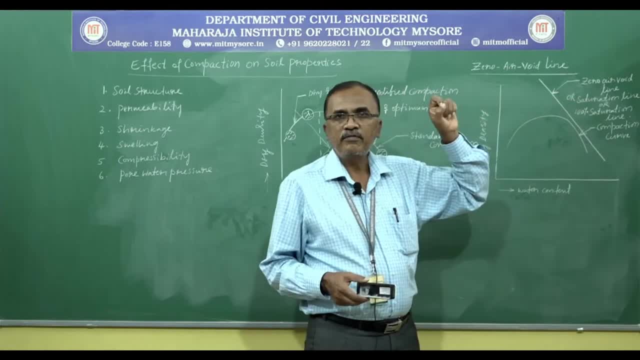 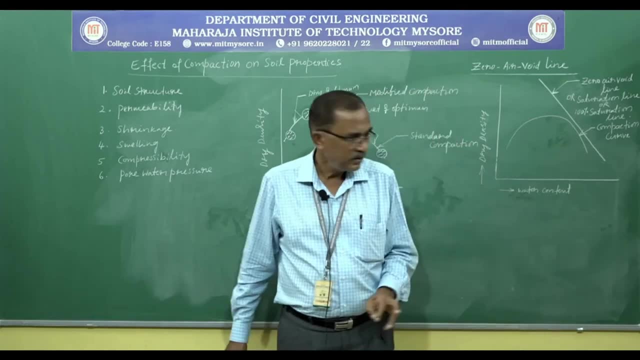 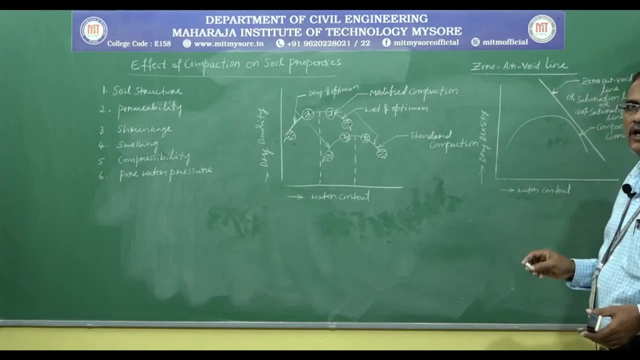 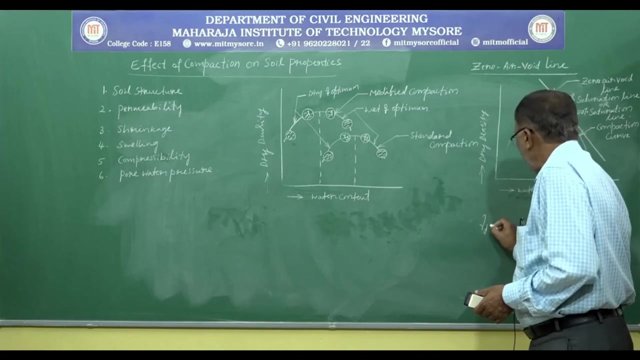 If you consider saturation line for other than 100 percent saturation line, this line will cross cross the compaction curve. So this, this die density corresponding to zero air void line for various water content, can be calculated By using the relation we have: gamma d is equal to g divided by 1 plus e into gamma w. also we have 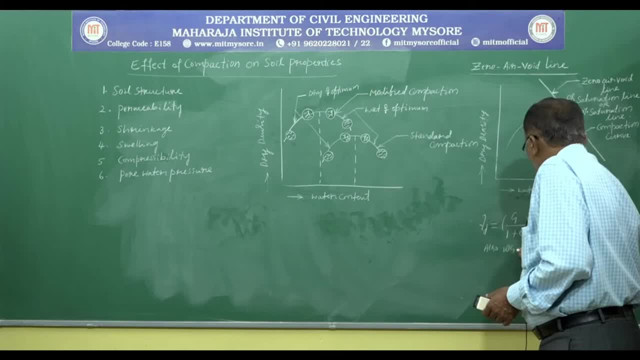 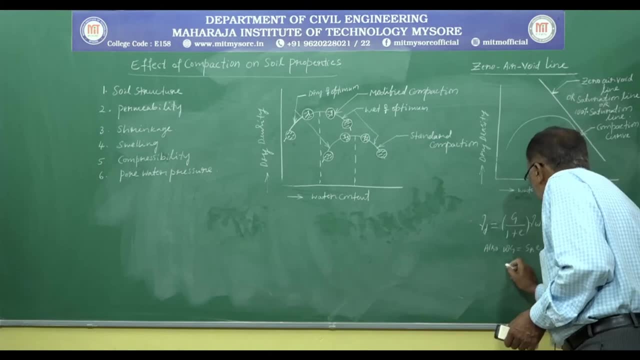 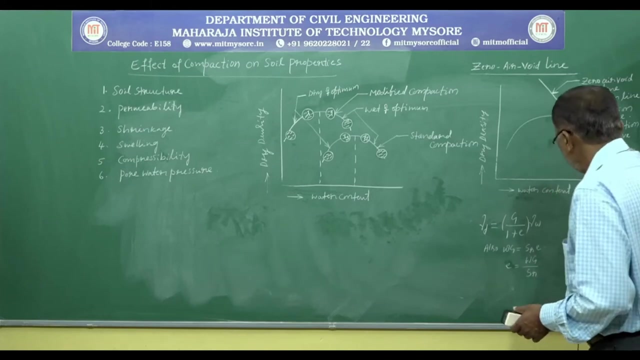 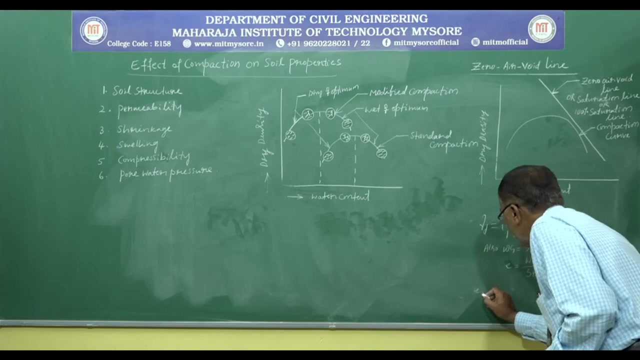 w g is equal to s r into e. therefore e is equal to w g divided by s r. If you substitute e here in the above equation, that is, gamma d is equal to g divided by 1 plus w g divided by s r into gamma w. 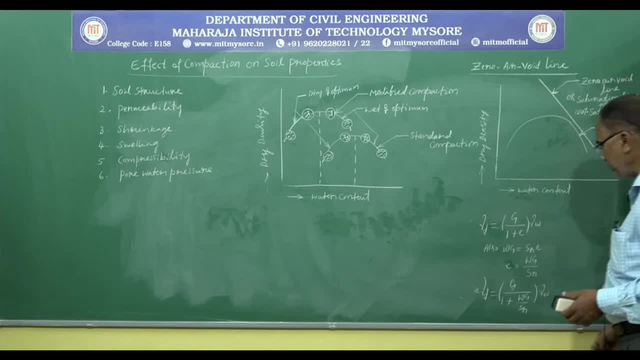 So this is the equation means it is gamma d z d a b. So this is the equation means it is gamma d z d a b. So this is the equation means it is gamma d z d a b corresponding to zero air void. in this equation, if we substitute, sr is equal to one hundred percent. 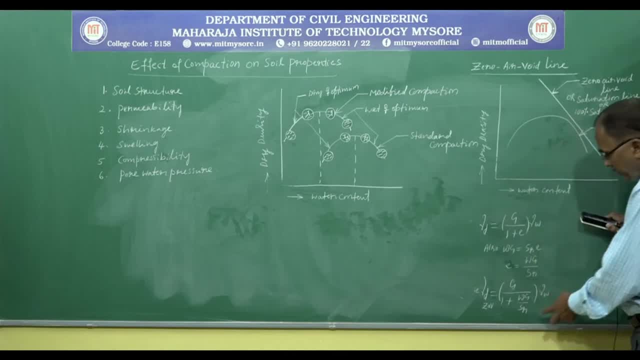 saturation means zero air void. we will get gamma d corresponding to zero air void. here the water content will be the water content selected for various trials of compaction. so as a result, we will get the gamma d. with the increase in water content there will be decrease in the gamma dzav. 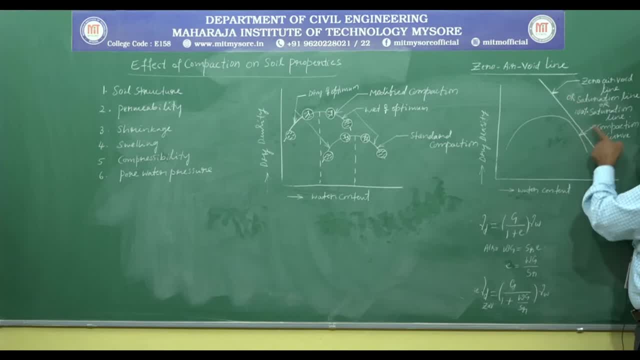 and finally the line will be parallel to the wet of the optimum curve. again, suppose, if you want to draw the saturation line other than hundred percent, say about 80 or 90, here degree of saturation to be taken as for example, for 90 percent, here it is 0.9 for 90 percent it. 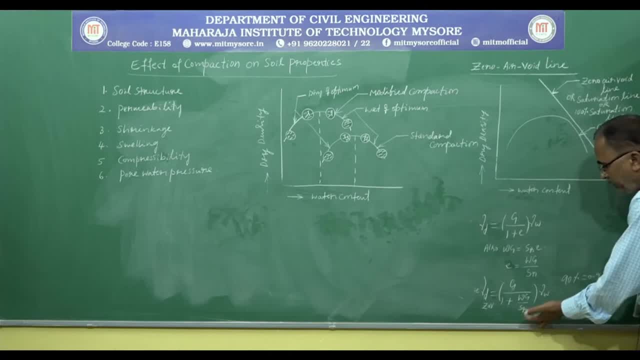 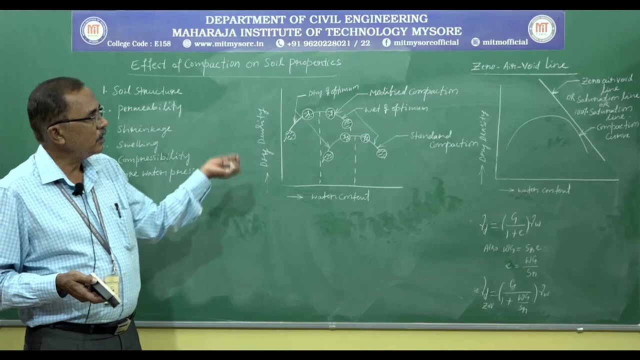 is degree of saturation is 0.9 and for 80 percent it is 0.8. like that, we can obtain the saturation line corresponding to 90 percent, 80 percent or whichever the percentage we want for all practical purposes, along with the compaction curve. 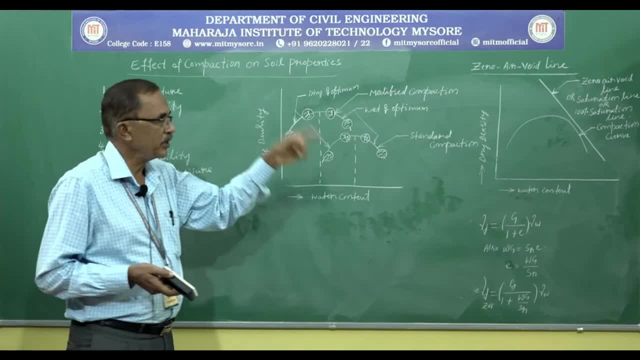 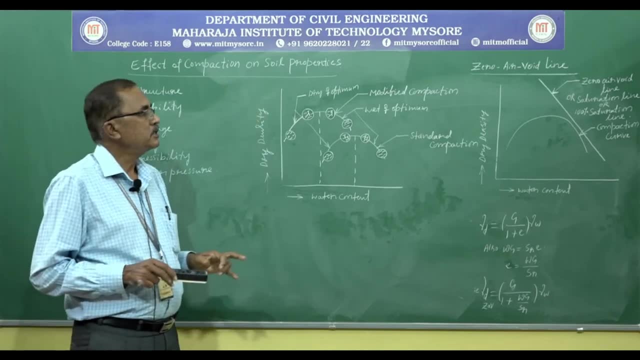 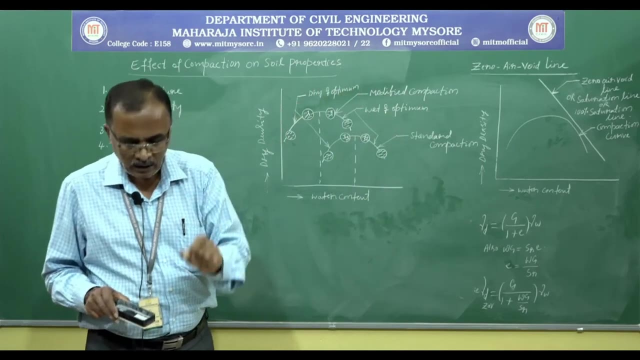 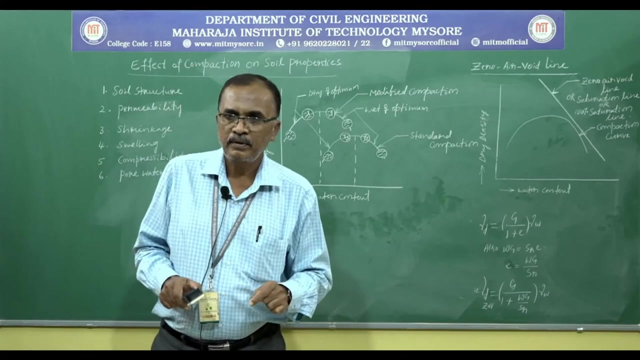 we also obtain or we also plot the zero air void line or the saturated line. this is about the zero air void line. it is a theoretical concept. zero air void line is a theoretical concept because it is highly impossible to reduce voids to zero, but still, for all important practical purposes and for all purposes, 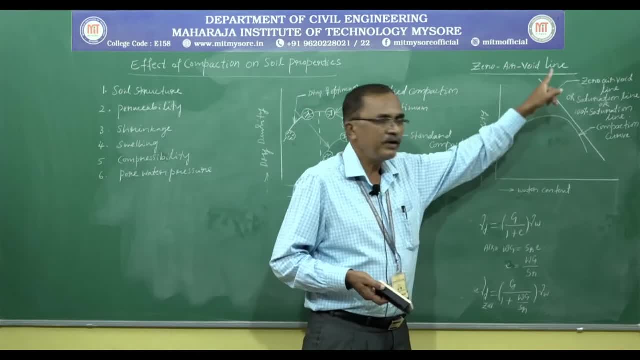 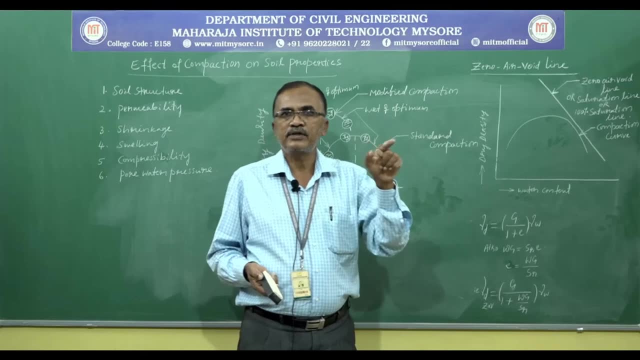 it is a theoretical concept because it is highly impossible to reduce voids to zero. we assume, after reaching to the optimum level we reach, that we have reached. we have achieved the hundred percent removal of air voids and consider the degree of saturation is equal to the zero. 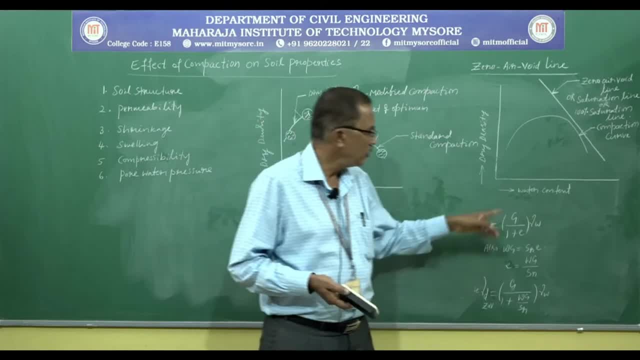 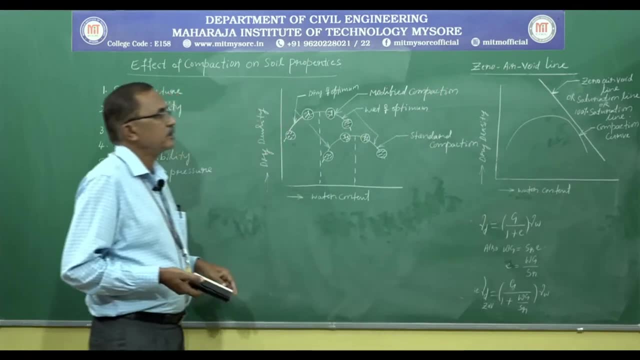 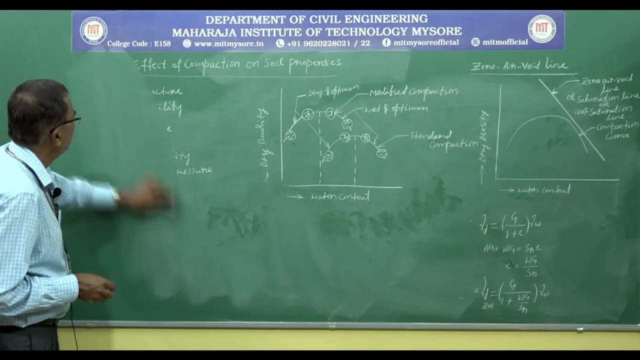 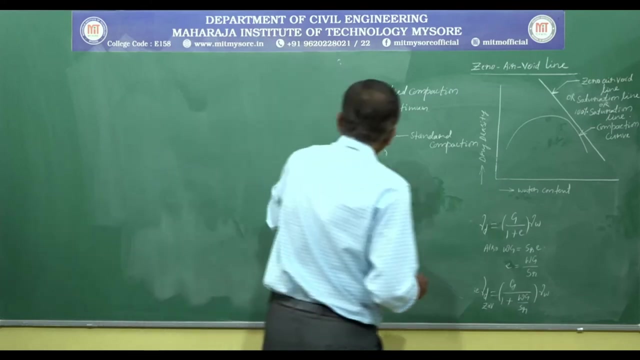 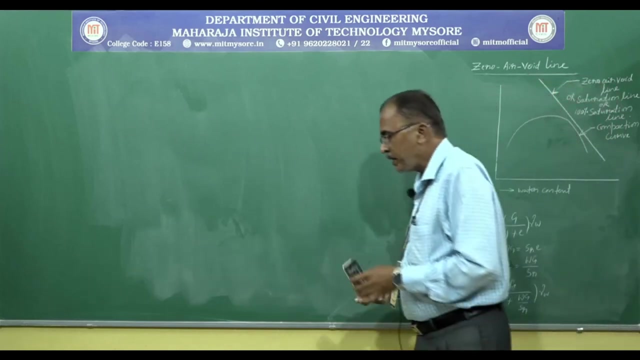 air voids and take will take a degree of saturation as one and obtain gamma d corresponding to zero air void line, and like this we can obtain the, the line or curve. we can obtain the given level of saturation, andв. but when we don't, alright, what we have done to destroy air void line is the reduction of. 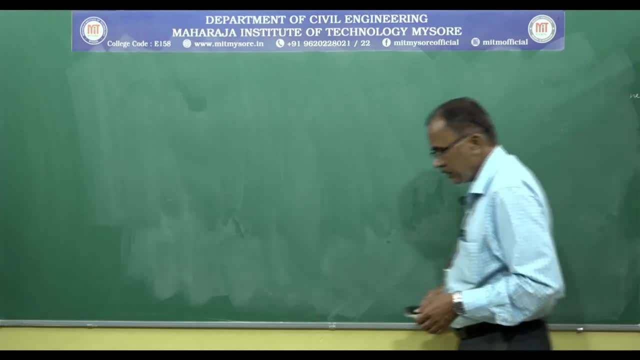 foam ratio during the total de absolution and with the help of neutron stellar number of Ki- slots, given sheets, and we get a solution for this question. So we are then cultured to first want to know that the time OD value will be 0 ate. 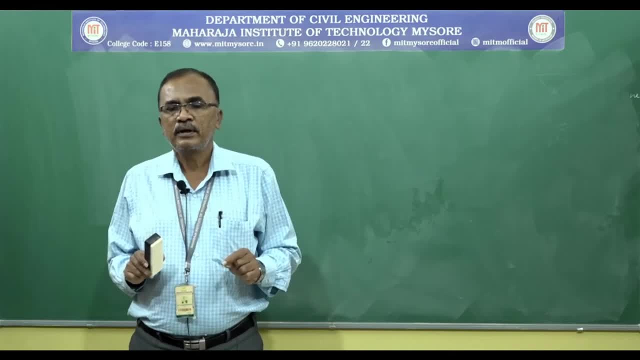 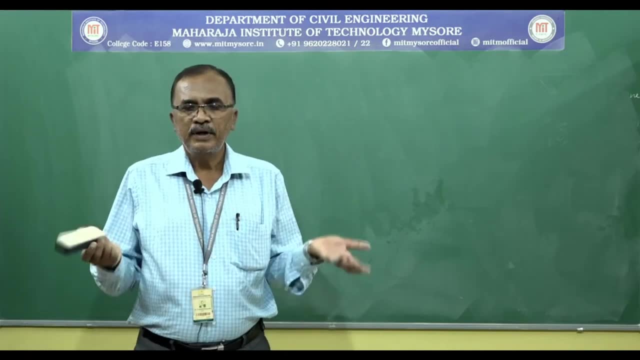 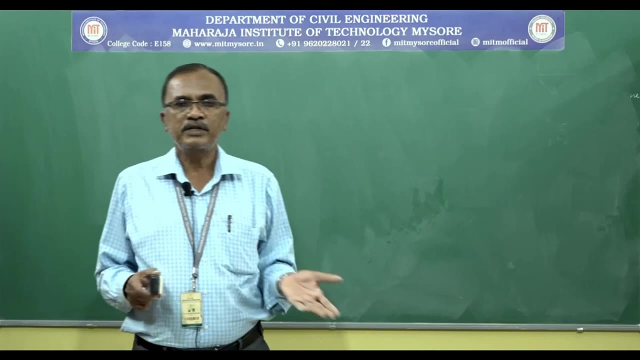 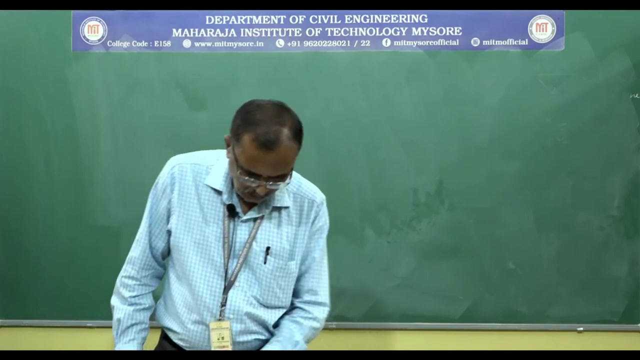 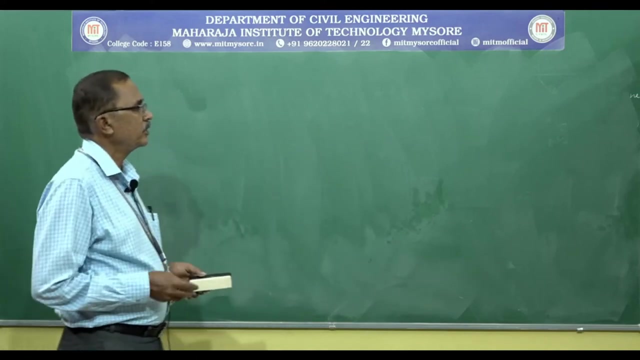 the dry density- water content relation and with the help of dry density and water content relation, we can easily understand the various concepts. concepts say, for example, it is the effect of factors affecting compaction, or effect of compaction on properties, and so on. so let us consider another important topic. it is laboratory compaction. 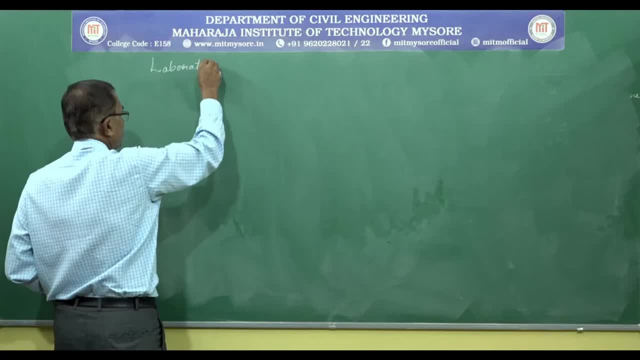 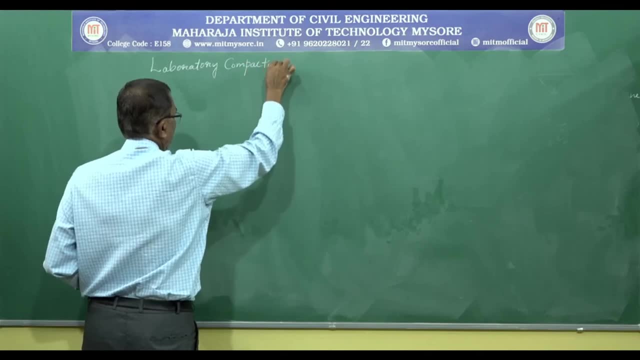 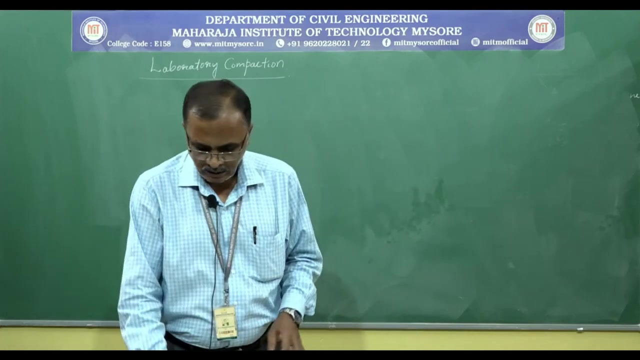 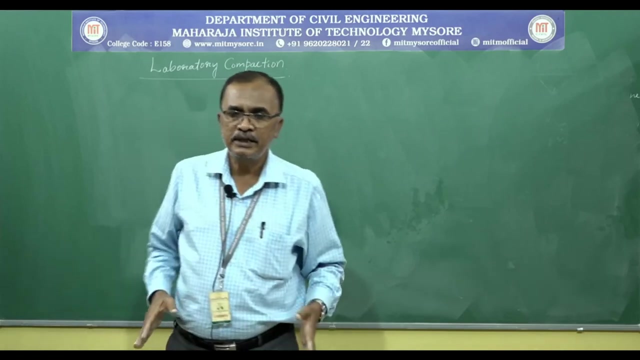 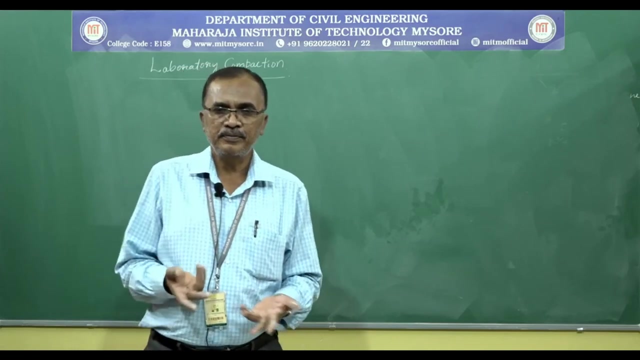 we know the objective of compaction. we know the objective of compaction. the very objective of compaction is to achieve the dry density, or density. purposefully. we increase the density to enhance the engineering properties. in turn, we will increase the shear strength repeatedly. i am using this so that that is. 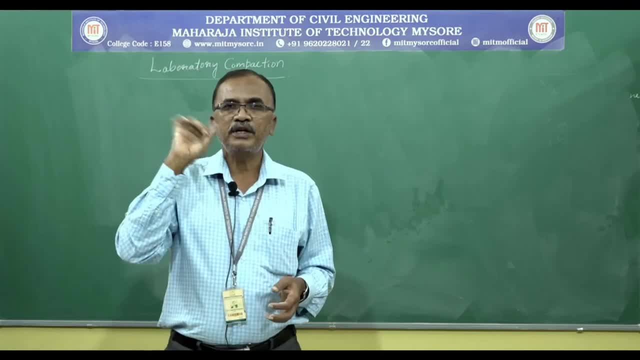 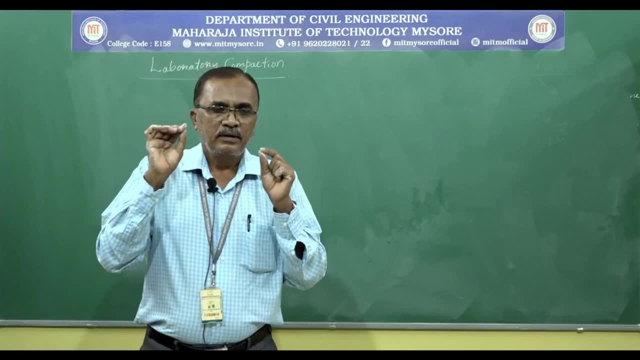 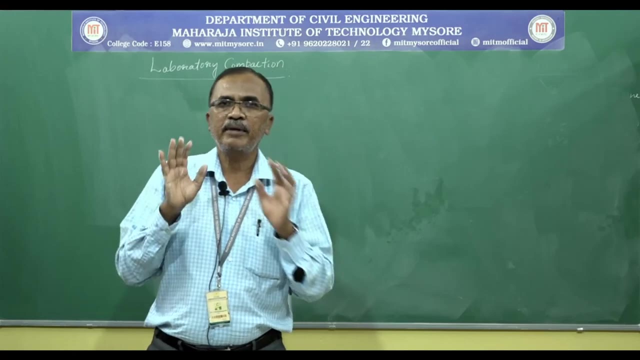 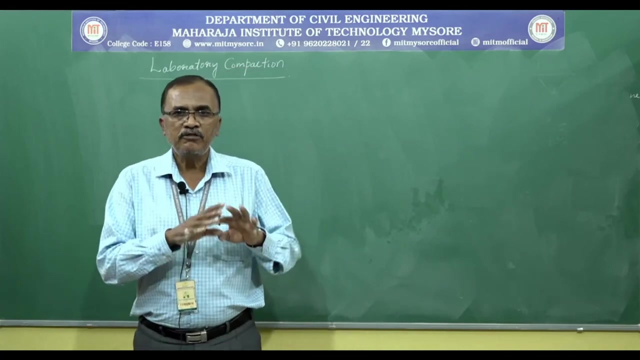 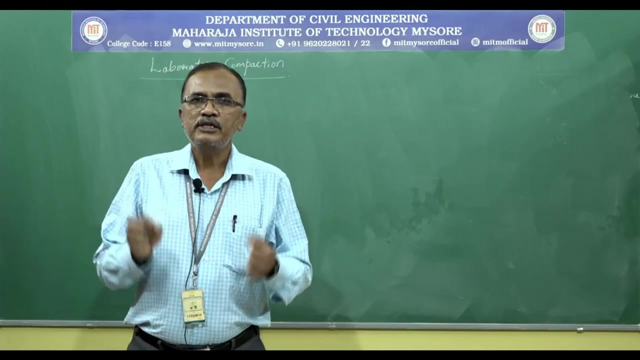 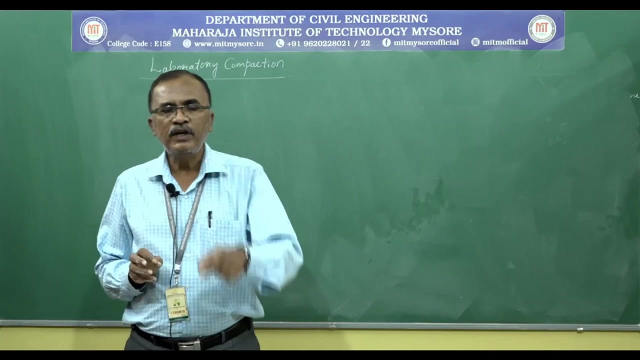 this objective and importance should be registered in your mind. compaction characteristics: we know compaction characteristics are optimal moisture content and maximal dry density. in the field, because of worst extent of soil, both in the longitudinal direction as well as lateral direction, it is very difficult to obtain compaction characteristics, but in the field we have to. 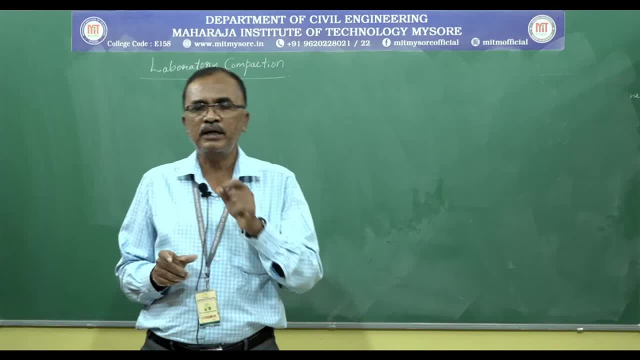 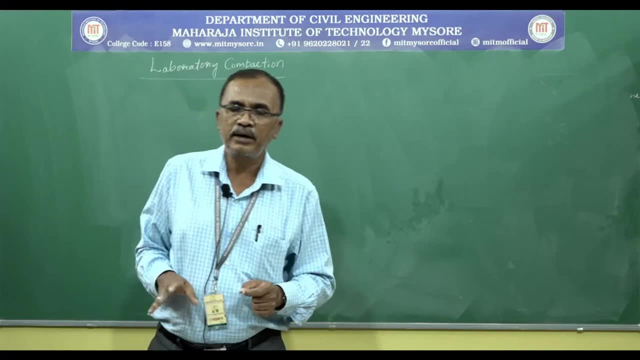 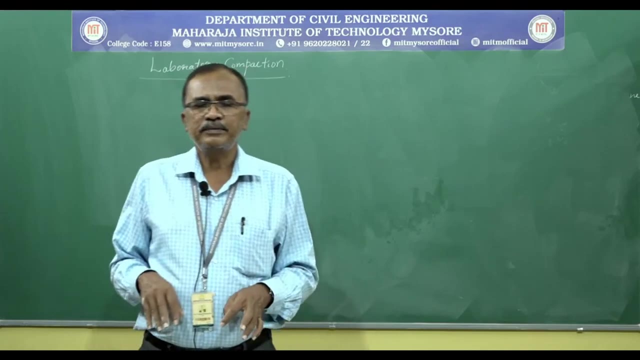 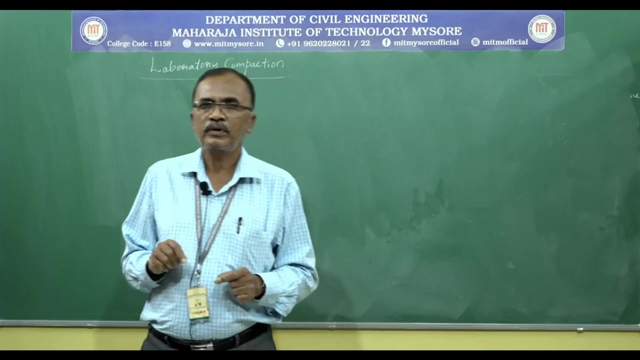 control the compaction. controlling compaction is nothing but uh: maintaining the temperature, danization, the required moisture content and importing the required mechanical effort. It leads to increase in the density For every soil to be used for construction purpose to be tested in the laboratory for their compaction characteristics. Under controlled condition in the laboratory depends upon the requirements. Requirements means whether we require more compacted soil or normally compacted soil. We decide the test- normal test or modified test. We obtain the moisture content and corresponding dry density and we take those compaction characteristics across the field and there we. 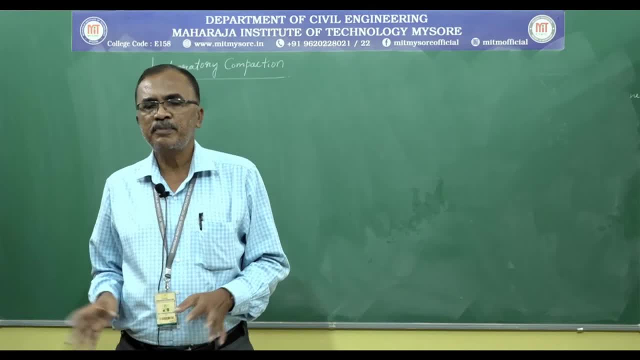 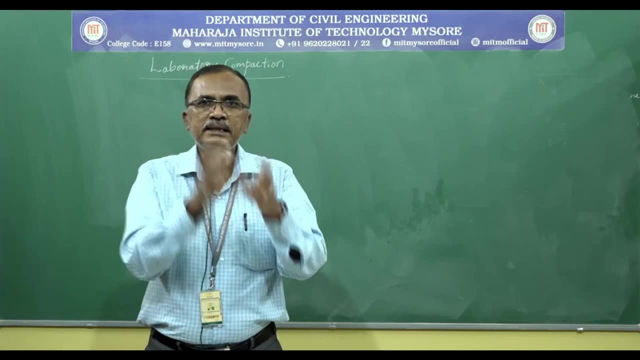 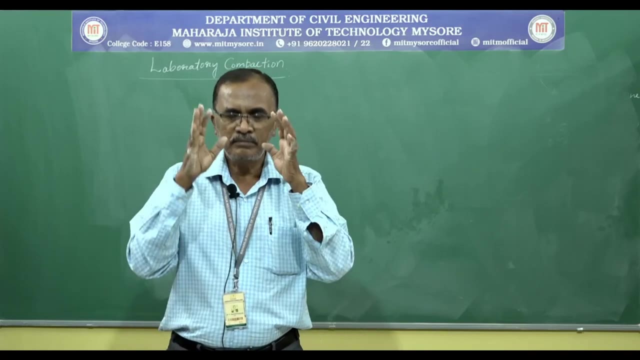 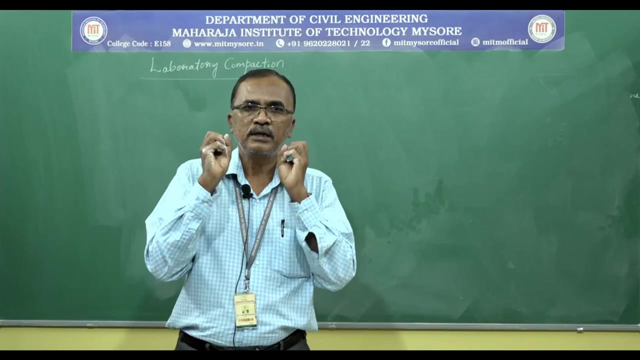 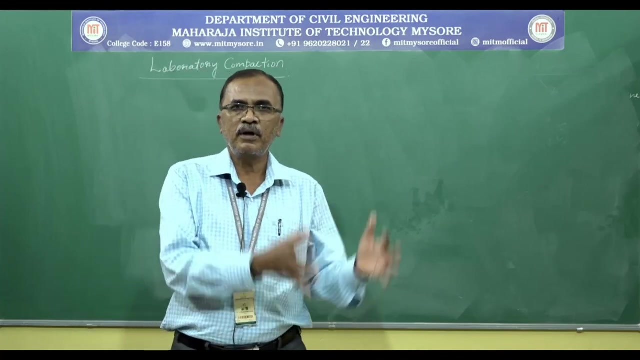 adopt the same to achieve the required density. This process is known as compaction control means at the site, before taking up construction. it is customary, it is mandatory nowadays, to know the compaction characteristics of soil. in order to achieve the desired compaction characteristics, First we bring soil- small quantity of soil- to the laboratory. 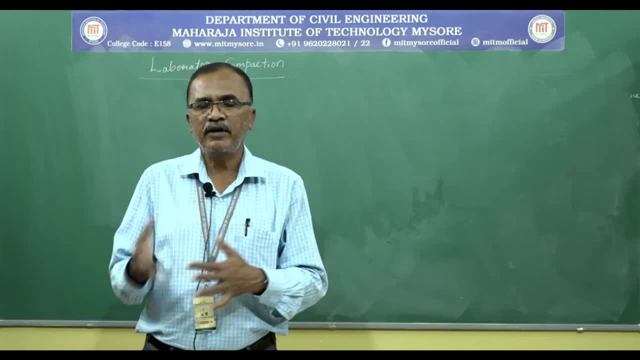 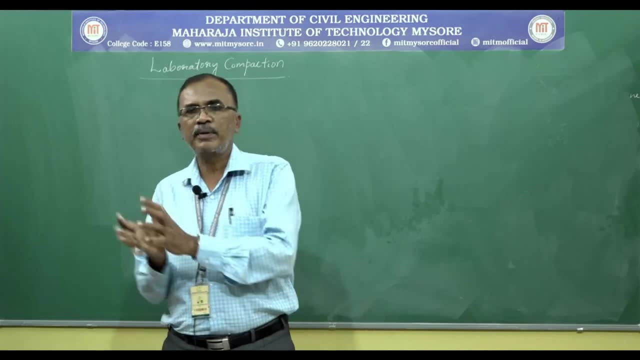 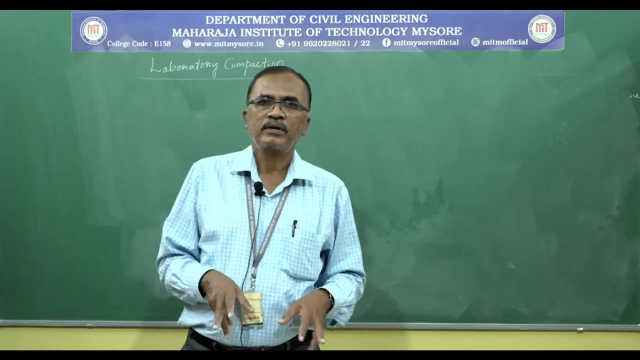 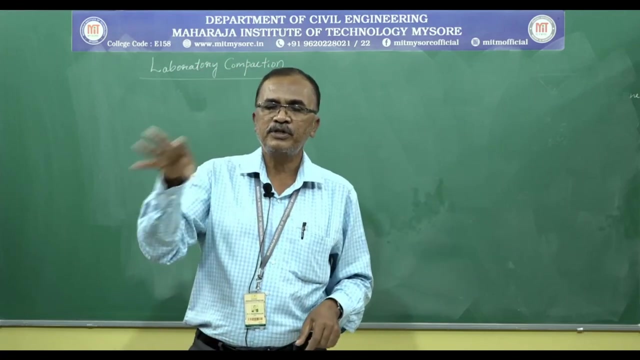 In the laboratory. we conduct the compaction test as per the requirement and we obtain the compaction characteristics and the same compaction characteristics we take into the field. there we again. we achieve the compaction till we reach to these. compaction characteristics means the water's optimum moisture content and the up to dry densities, that the maximum dry density 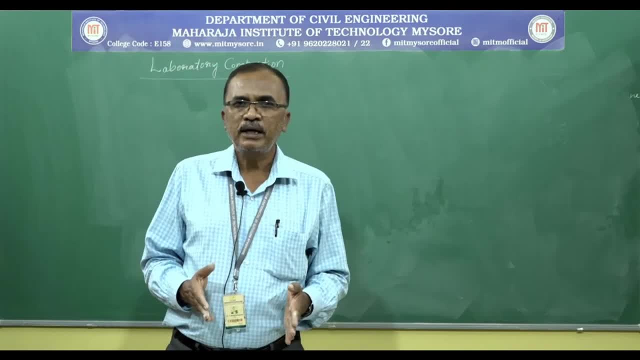 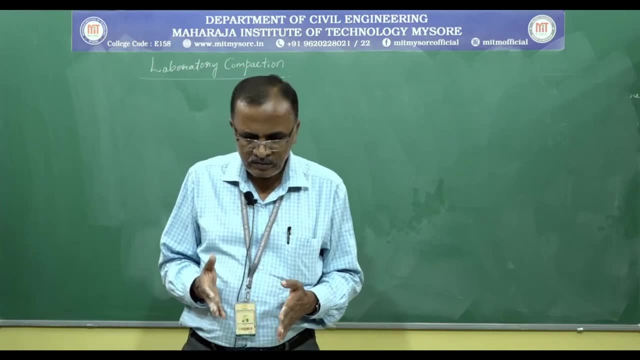 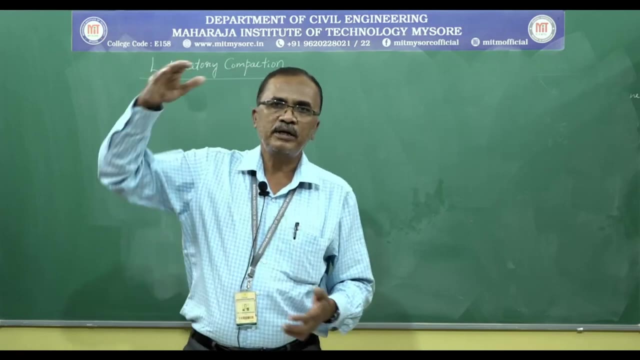 This has to be done for every project. particularly this is for when we go for the embankment. During embankment construction. rarely we get the required soil at the site. Generally we have to get the soil from the away- little away from the construction site or far. 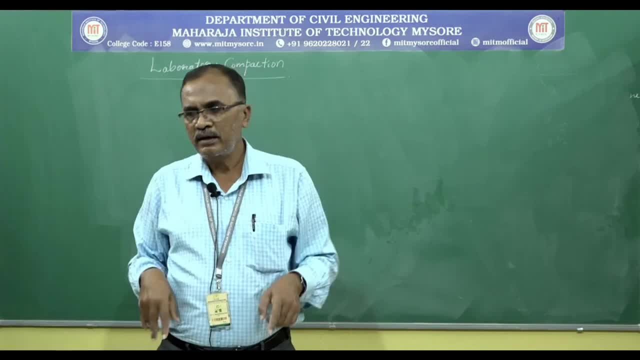 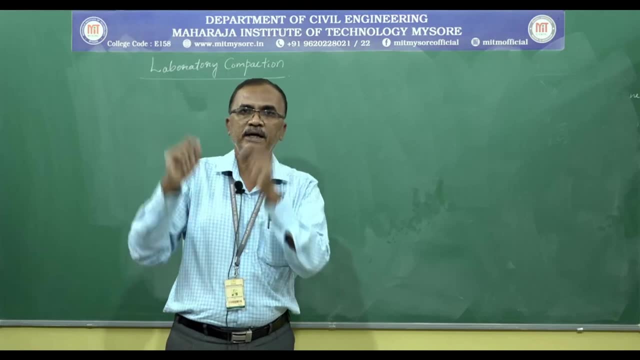 away from the construction site and we identify the area, and that identify area is known as borrow area. From the borrow area first we bring the soil sample to the laboratory. In the laboratory we conduct the compaction test and we obtain the compaction characteristics. 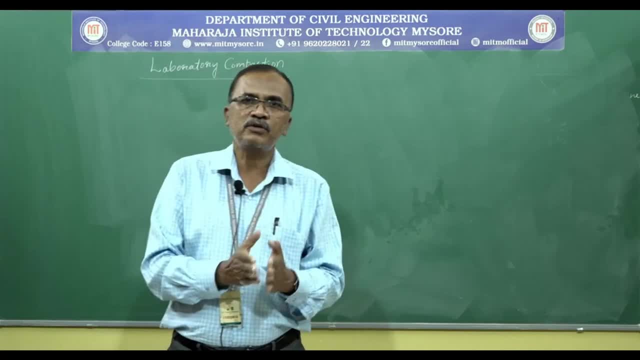 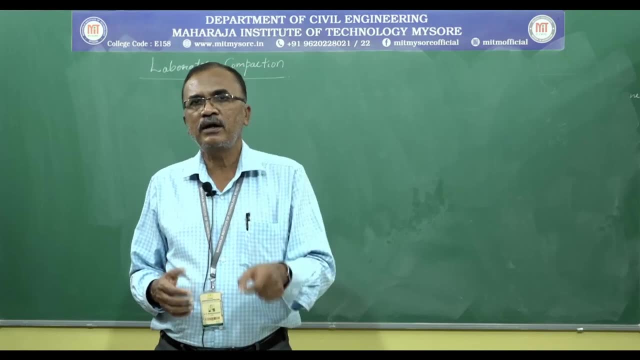 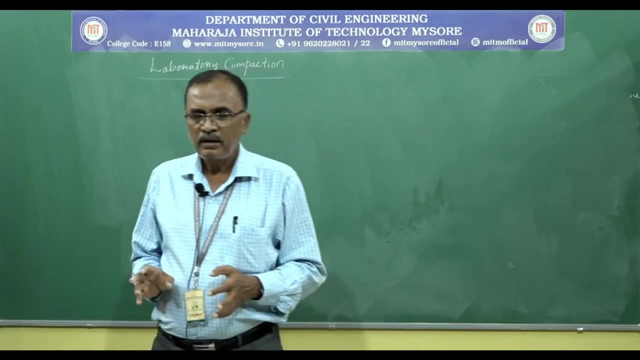 These compaction characteristics will be considered as a reference. while doing compaction in the field, And after compaction of each stretch, we check for the added water and achieve density. If any of these is not sufficient or not reached to the required value, then we alter the, we increase. 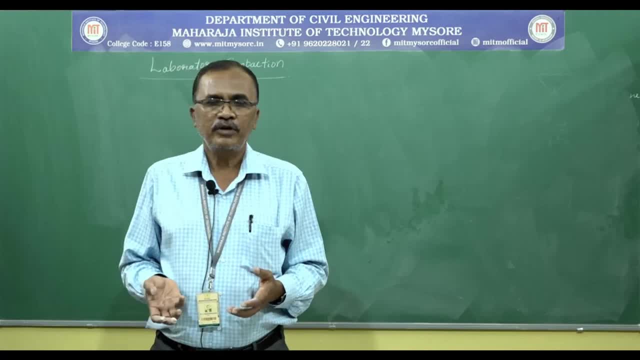 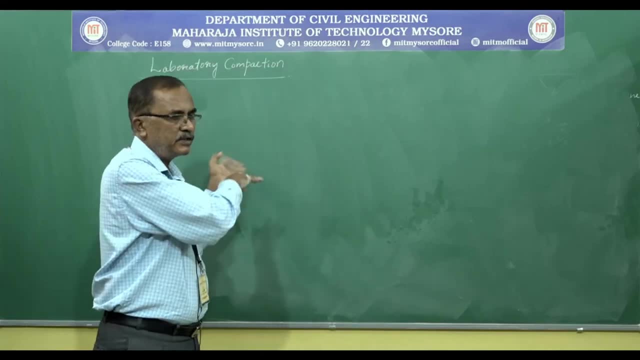 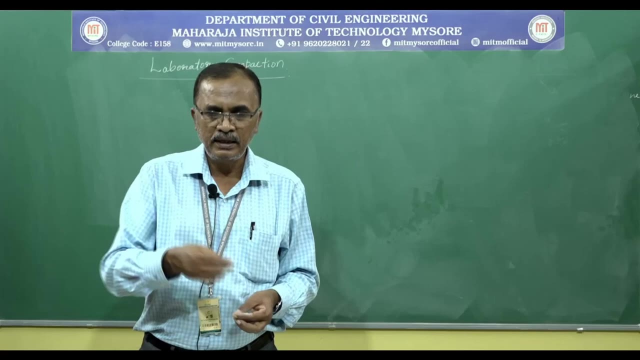 the water content or we increase the, the compact the effort. For that we have to conduct the compaction test first in the laboratory. then these results will be transferred to the the field. So we will discuss this laboratory test again in detail in the next class.